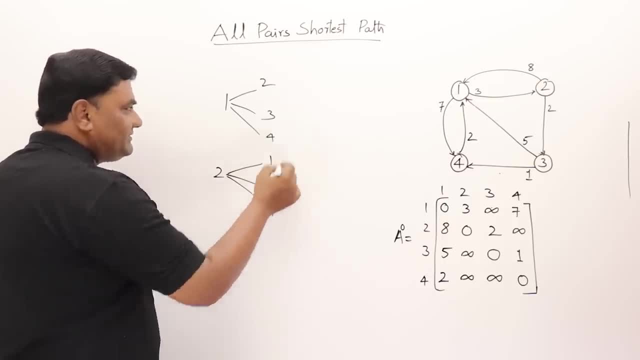 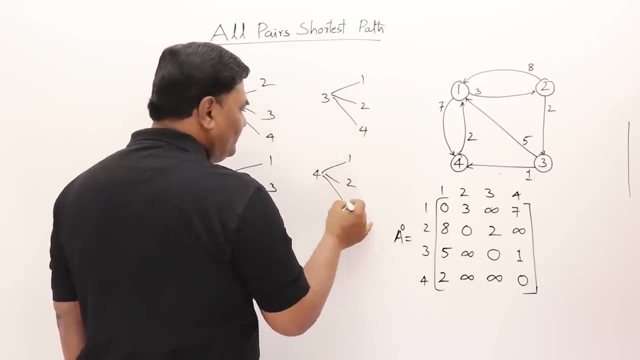 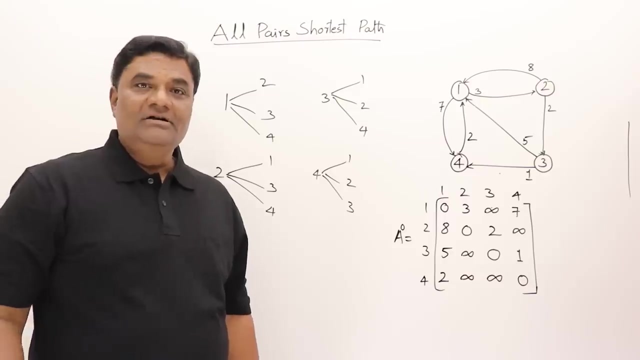 vertex 1 and 3 and 4.. Similarly, from 3 I should find a shortest path from 1, 2, and 4 to 1 and 3.. Similar to single source: shortest path. that is the Dijkstra algorithm. 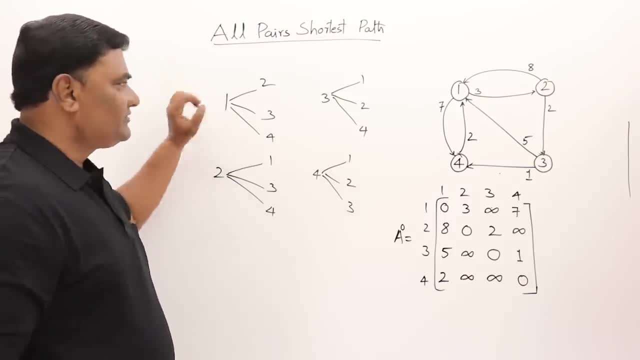 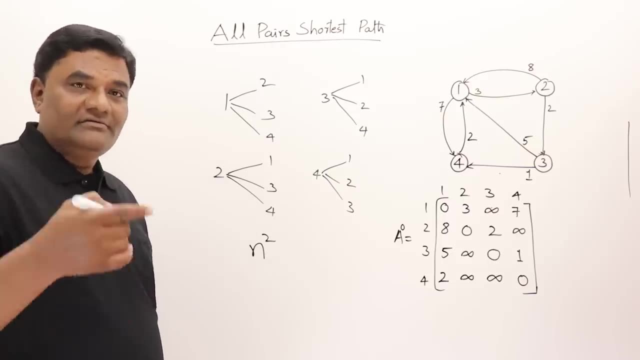 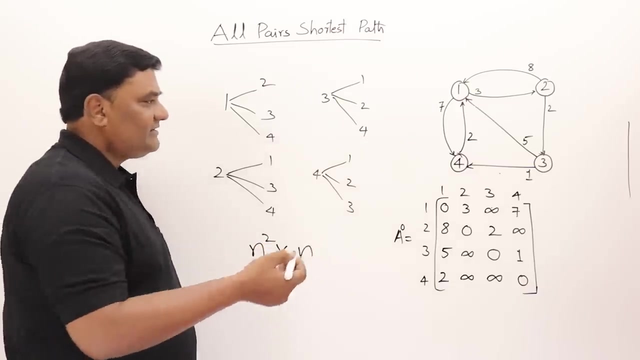 But deijkstra algorithm will find out the shortest path from one of the source vertex: dangerous Dijkstra dextra takes order of n square time. If I run dextra algorithm on all the vertices one by one, that is, all n vertices, then I can get the result. Yes, I can use dextra algorithm. 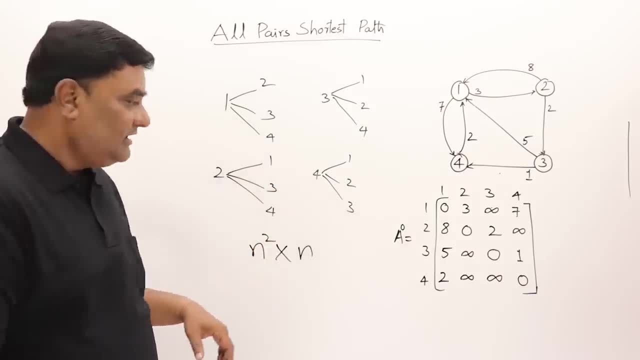 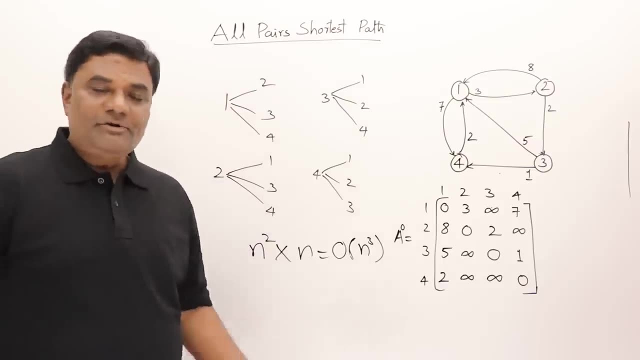 for solving this problem for all n vertices one by one, and for each vertex it will take n square time and the time will be order of n cube. So this problem can be solved using greedy method also. but let's now see how we can apply dynamic programming for solving. 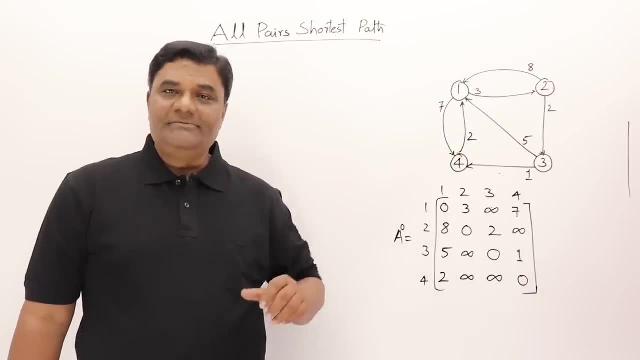 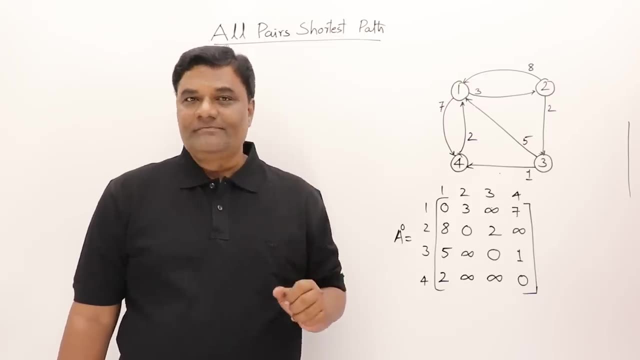 this problem Now how the problem can be solved using dynamic programming. Dynamic programming says that the problem should be solved by taking sequence of decision. In each stage we will take a decision. So what decision I have to take? Let us see. See if I have. 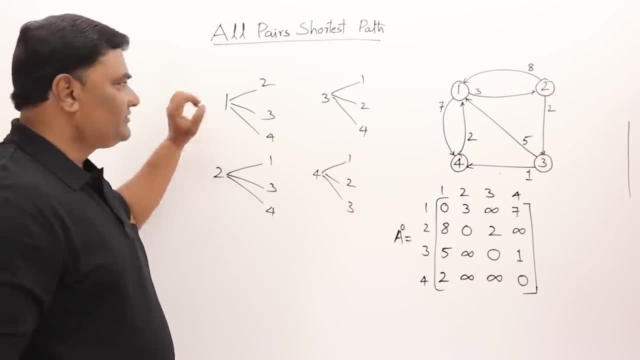 But Dijkstra algorithm will find out a shortest path from one of the source vertex and theiutraalgorithm, goddamn, will find out short paths from one of the source vertex evidence. and diktraalgorithm will find out a shortest path from 1 too. This screen will show 2 and 3, but again. 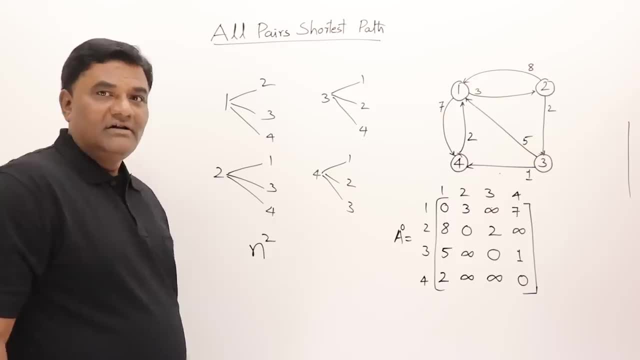 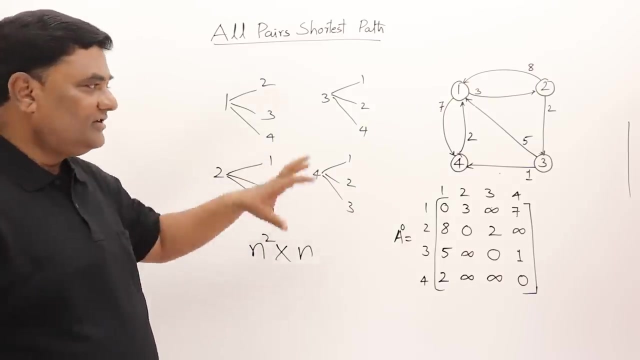 dextra takes order of n square time. If I run dextra algorithm on all the vertices one by one, that is, all n vertices, then I can get the result. Yes, I can use dextra algorithm for solving this problem for all n vertices, one by one, and for each vertex it will take. 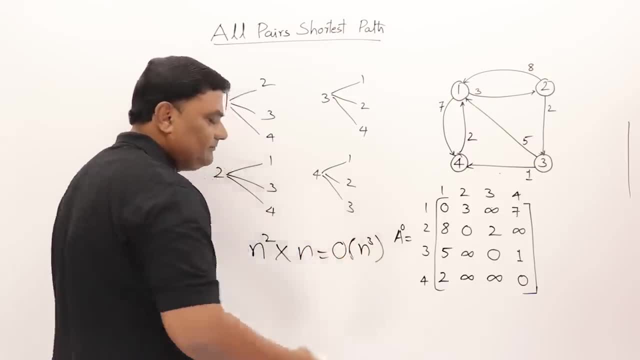 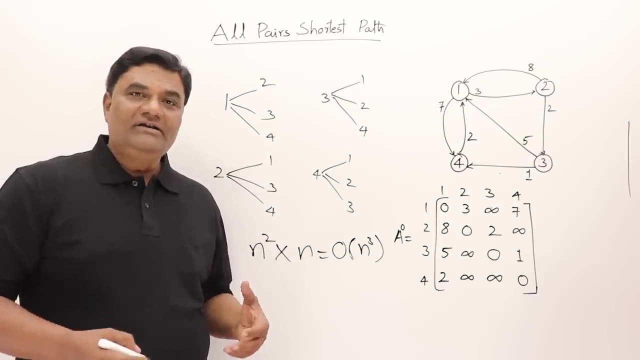 n square time and the time will be order of n cube. So this problem can be solved using greedy method also. but let's now see how we can apply dynamic programming for solving this problem. Now, how the problem can be solved using dynamic programming. Dynamic programming. 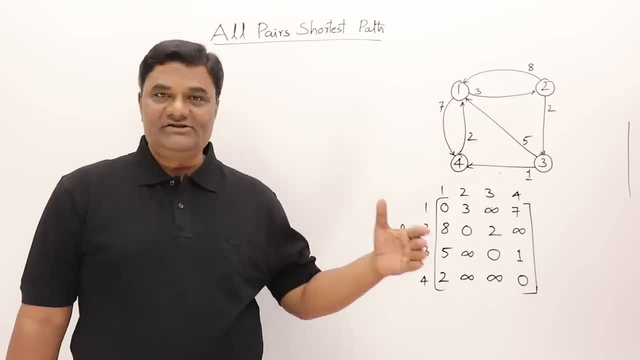 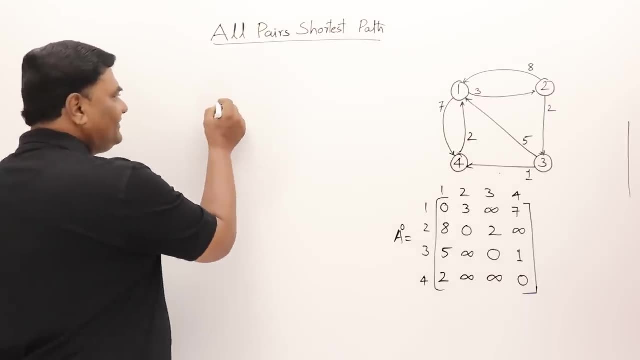 says that the problem should be solved by taking sequence of decision. In each stage we will take a decision. So what decision I have to take? Let us see See if I have to find a shortest path between vertex one to two, So there may be a direct edge path. 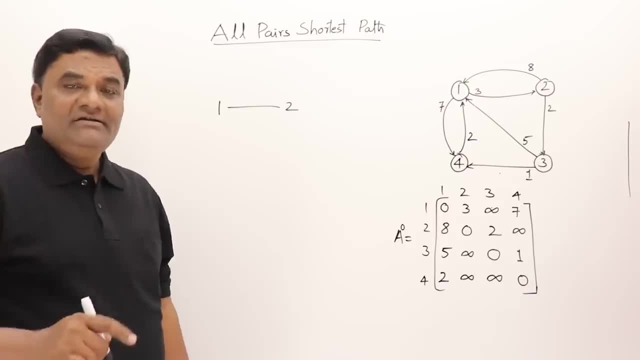 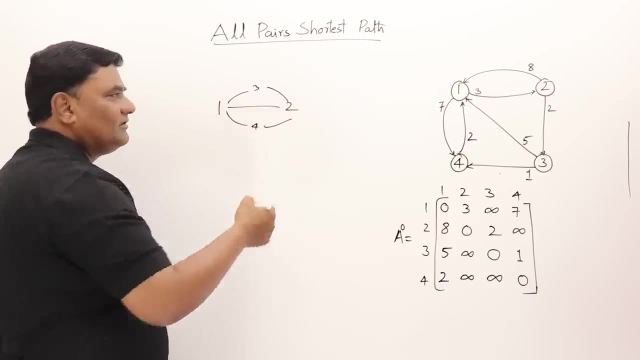 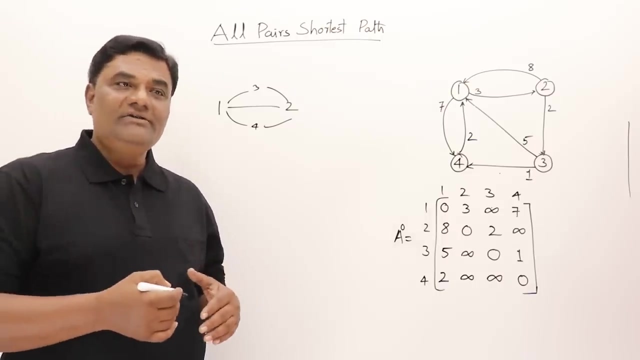 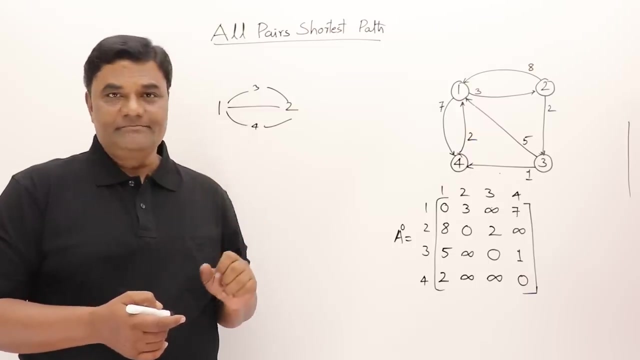 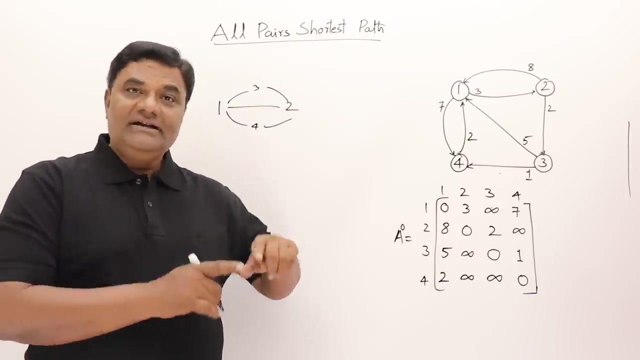 from one to two, also like here you can see, or may be there is a shortest path between vertex one to two. So there may be a direct edge path from one to two, also like here you can see, or may be there is a shorter path going via vertex three, or it may be going via vertex four. So in this way I have to check or decide whether a shorter path is going via some other vertex. So I will start selecting the middle vertex as vertex one, So I will find out first whether there is a shorter path between all the pair of vertices going via vertex one, then via vertex two, and so on. 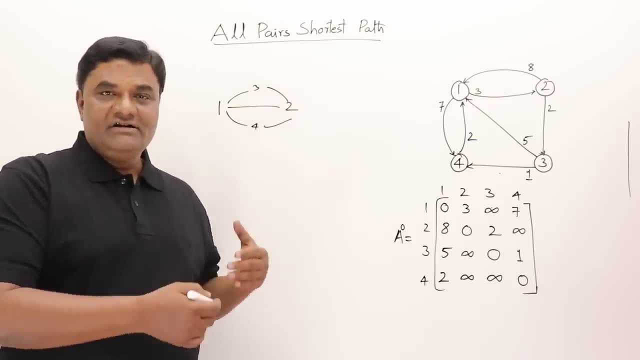 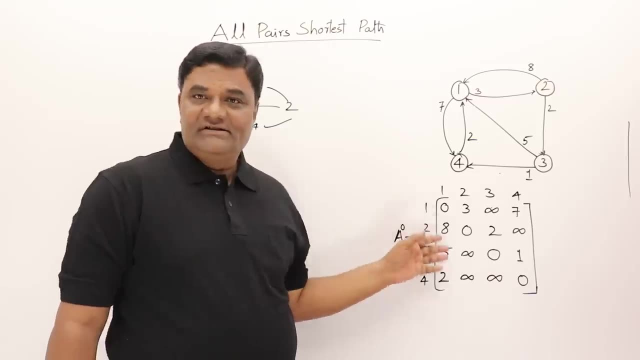 So this is how we can take decision, or sequence of decisions. So how this can be done, This can be done by just cloning matrices. Let me explain you with this: adjacency matrix, see here from one to one or two to two, then through: 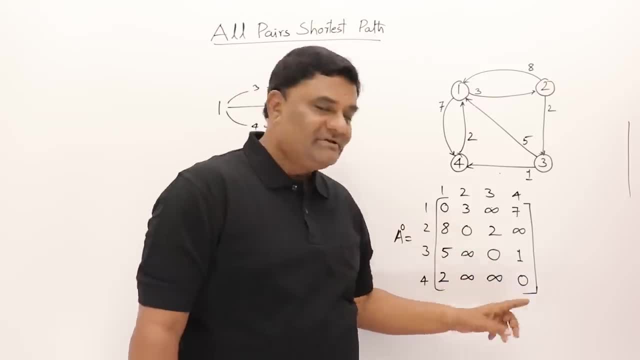 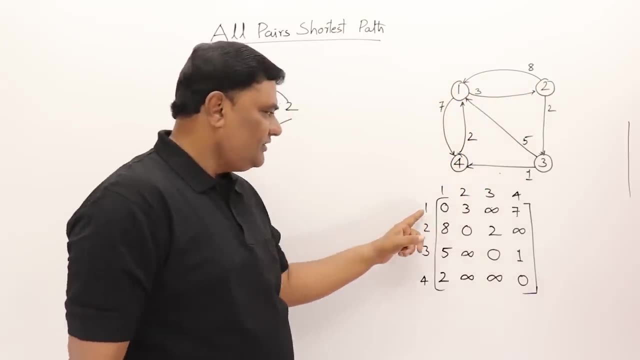 four to four. there is no edge. that is why all these are zeros means there is no edge we can have. Then there is an edge going from one to two. so one to two, the cost of an edge is three. And similarly there is an edge going from two to seven. 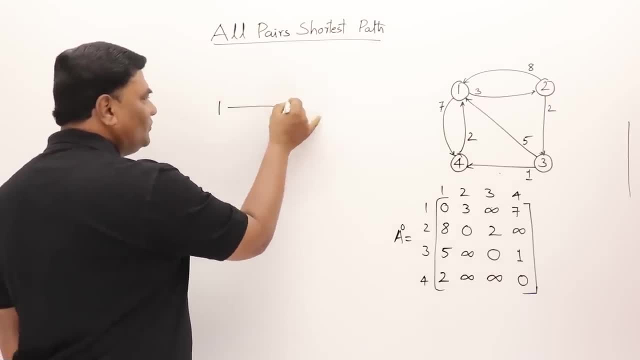 to find a shortest path between vertex one to two, So there may be a direct edge path from one to two also, like here you can see. or maybe there is a short path between vertex one to two, So there may be a direct edge path from one to two also, like here you can see. or maybe there is a 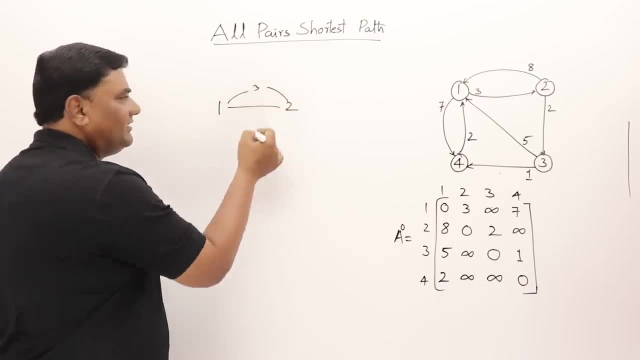 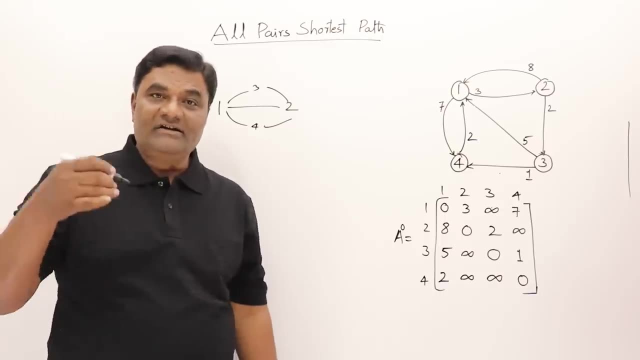 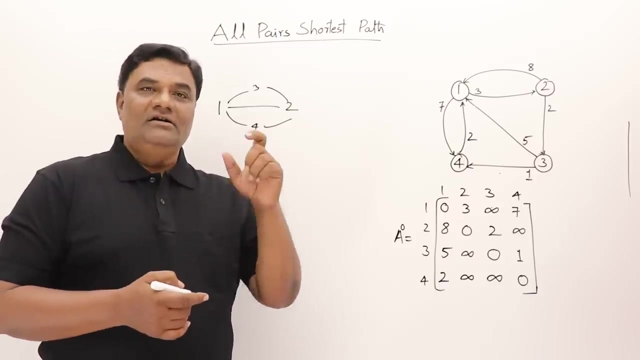 shorter path going via vertex three, or it may be going via vertex four. So in this way I have to check or decide whether a shorter path is going via some other vertex. So I will start selecting the middle vertex as vertex one. So I will find out first whether there is a shorter path between all the pair of vertices going via vertex one, then via vertex two, and so on. 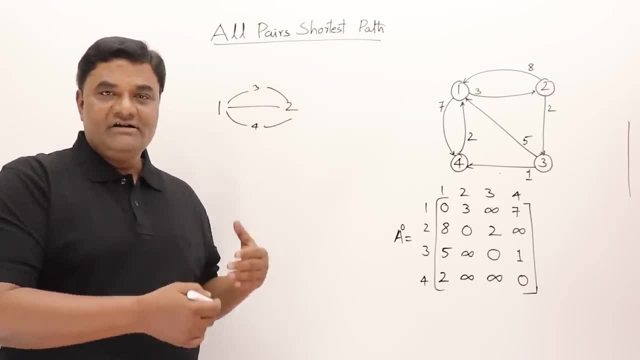 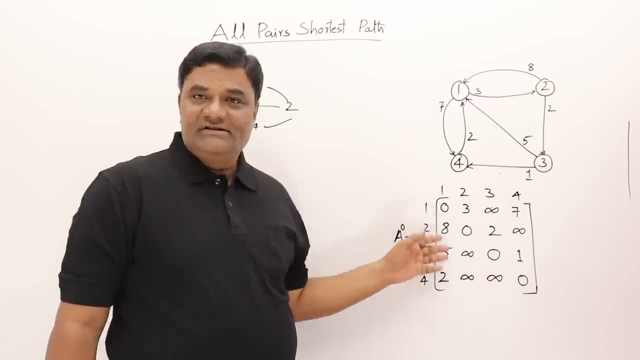 So this is how we can take decision, or sequence of decisions. So how this can be done, This can be done by just preparing matrices. Let me explain enough of this adjacency matrix. See here from one to one or 2 to 2.. four to four. There is no edge. That's why all these 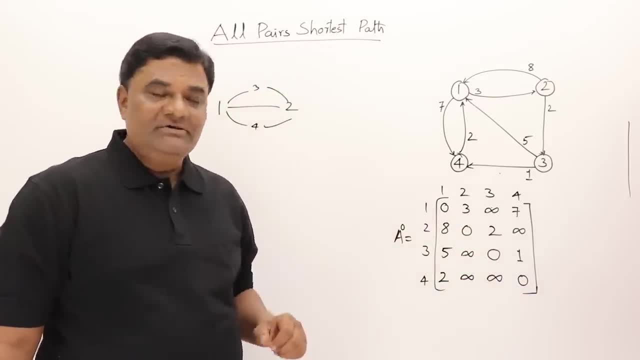 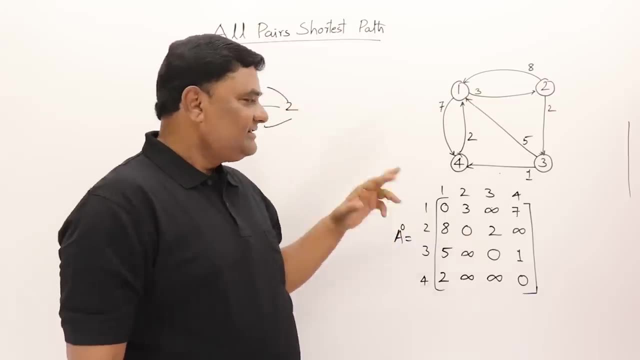 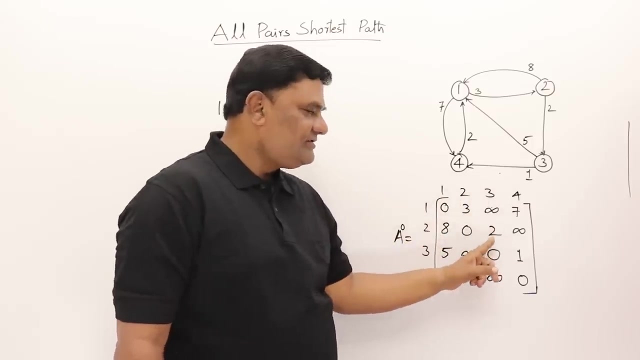 are zeroes, There is no edge possible, Loops are not possible. Then there is an edge going from one to two, So one to two, the cost of an edge is three. And similarly there is an edge going from 2 to 3, so the cost of an edge is 2. so 3, 2 to 3, the cost of an edge is 2 if there is no edge from 3 to 2. 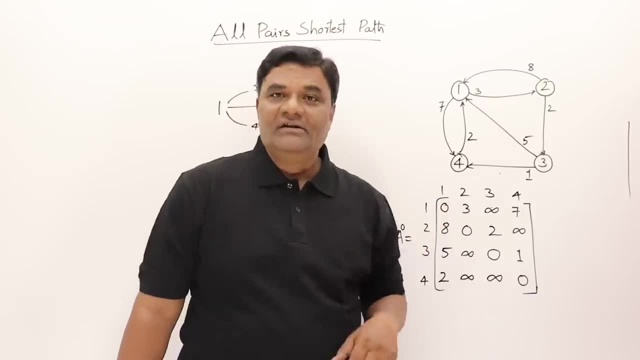 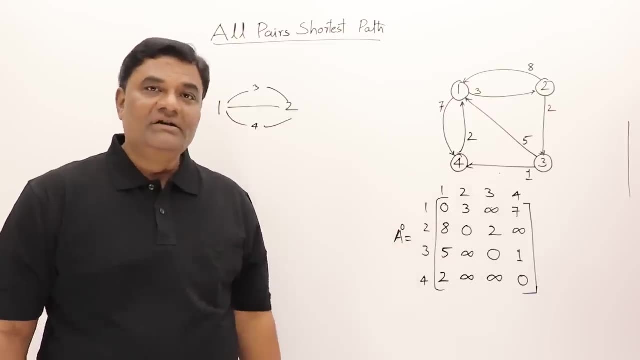 there is no edge, you see. so 3 to 2 is kept as infinity. in case of absence of any edge, we will take it as infinity, otherwise, for self loop, we will show them as 0. now, how we will solve this is: we will solve it by preparing matrices. so let us see how matrices can be prepared. 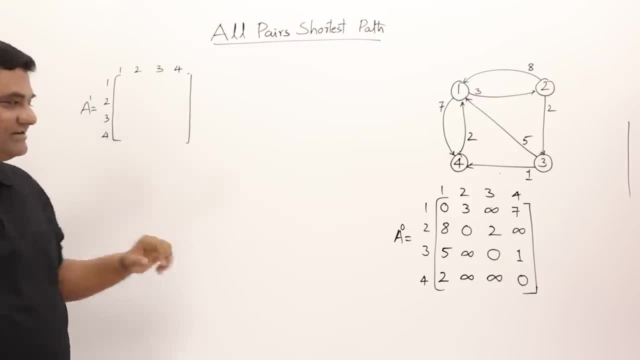 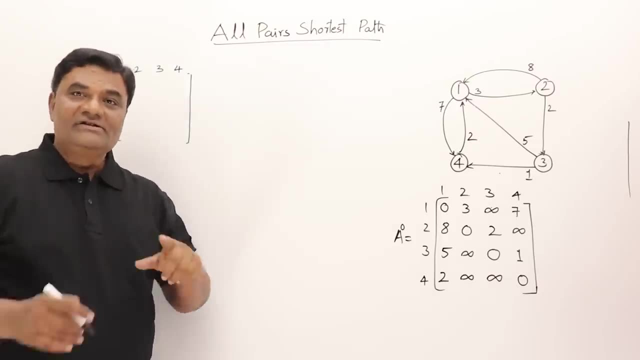 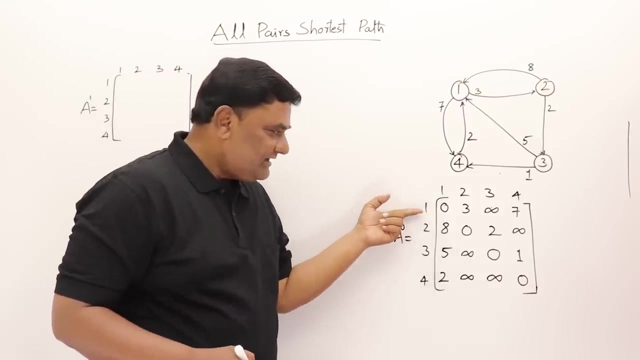 let us prepare a matrix for 1, a 1. see, this was a 0 original matrix. now here i am going to consider the intermediate vertex as vertex 1. so is there any better, shorter path going via vertex 1? so when i say vertex 1, then all the paths that belongs to vertex 1 will remain unchanged. so i should not. 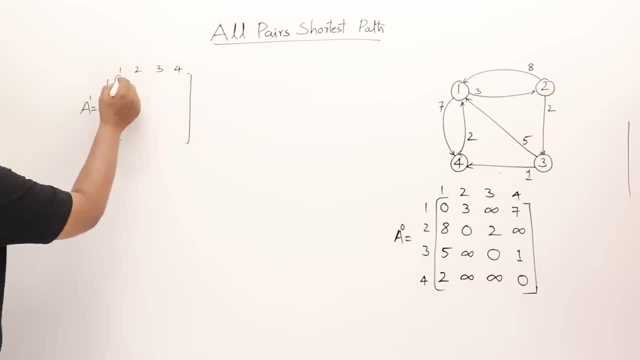 calculate them directly. i can take them here. so those values are 0, 3, infinity and 7, and these are 8, 5 and 2, so first row and first column already i have taken as it is. then what about the diagonals? there are no self loops, so i will fill those diagonals also. now remaining values i have to. 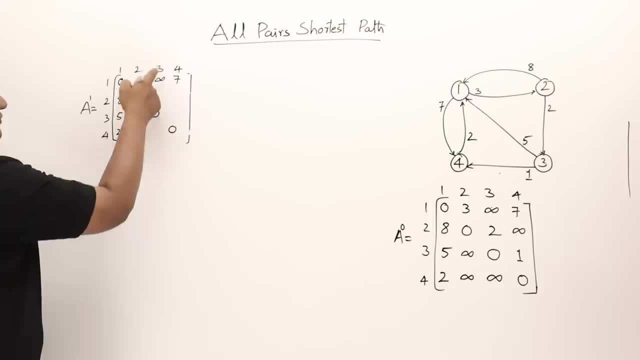 find out what are those. first, let us check this one that is 2 to 3. so how to get this value, how to check whether there is a shorter path via vertex 1 or not? so 2 to 3. i will take a 0 of 2 to 3. 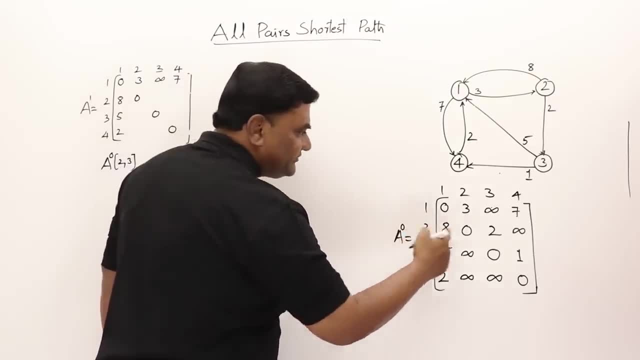 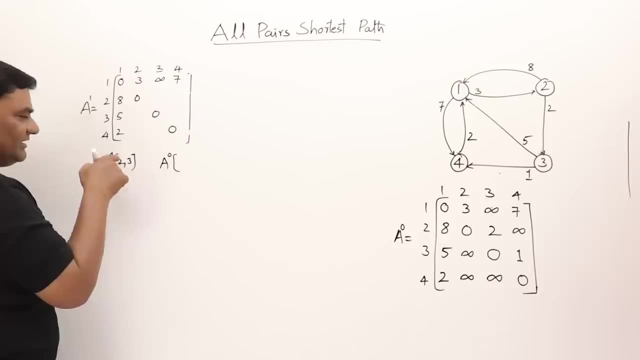 so what is there in this matrix? 2 to 3. so 2 to 3 is the shortest path going via vertex 1. so 2 to 3 is 2 and a 0 of now. in between i should include vertex 1, so 2 to 1 and 1 to 3 from those matrix. 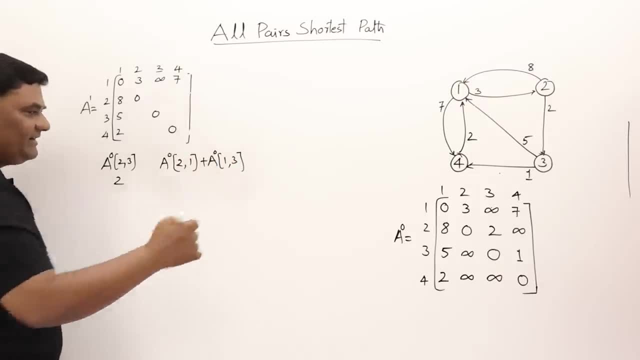 from that matrix 2 to 1 and 1 to 3. 2 to 1 is how much 8? 1 to 3 is infinity. so this is 8 plus infinity. this is infinity, only this is less. so there is no better path via vertex 1. 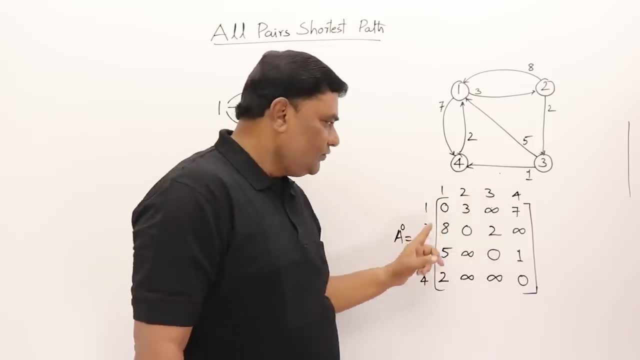 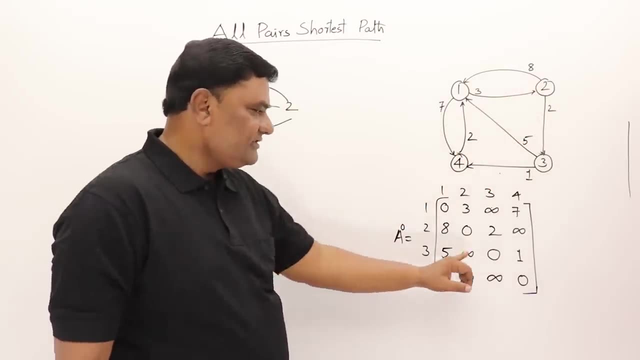 3. So the cost of an edge is 2.. So 2 to 3, the cost of an edge is 2.. If there is no edge from 3 to 2, there is no edge, you see. So 3 to 2 is kept as infinity In case of absence. 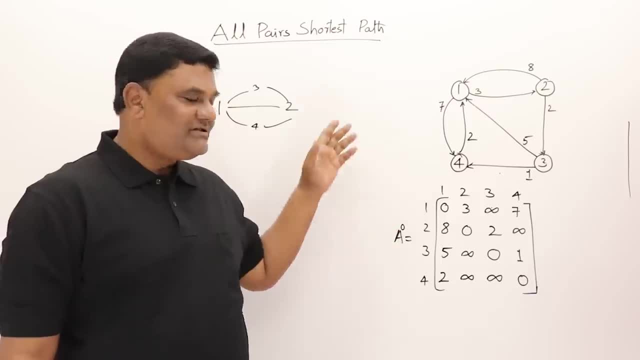 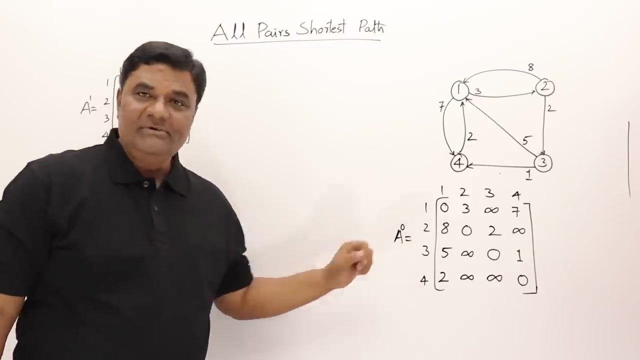 of any edge, we will take it as infinity. otherwise, for self loop, we will show them as 0.. Now how we will solve this is: we will solve it by preparing matrices. So let us see how matrices can be prepared. Let us prepare a matrix for 1, A1.. See, this was A0 original matrix. Now 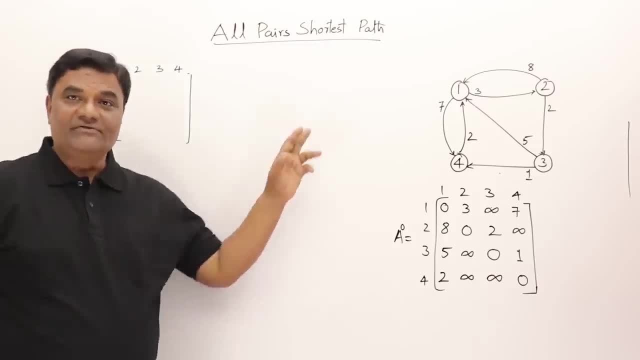 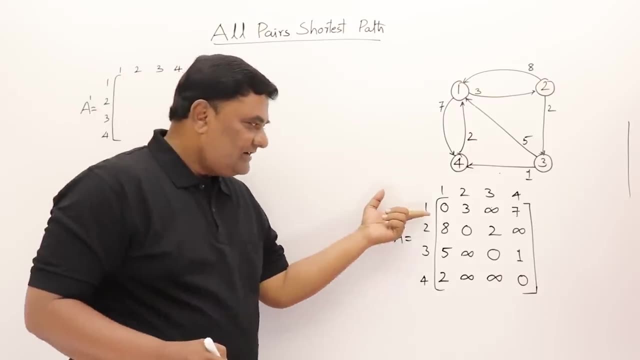 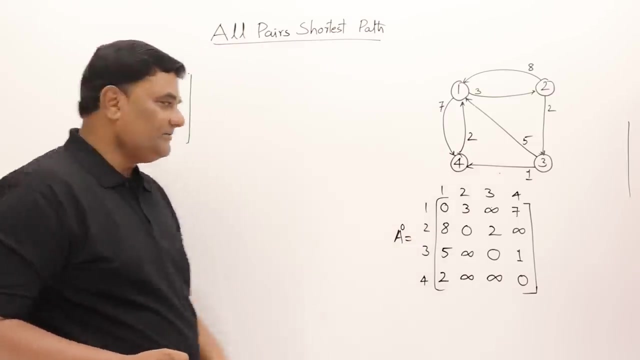 here I am going to consider the intermediate vertex as vertex 1.. So is there any better, shorter path going via vertex 1?? So when I say vertex 1, then all the paths that belongs to vertex 1 will remain unchanged. So I should not calculate them directly. I can take them. 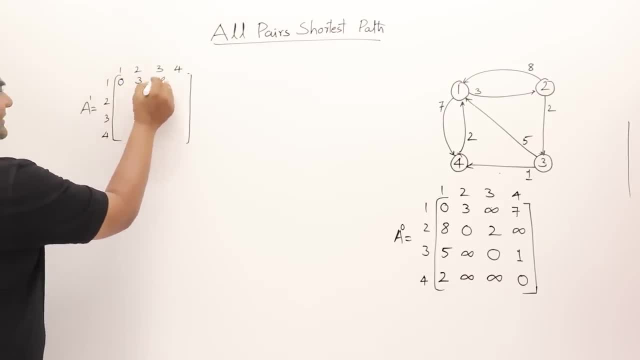 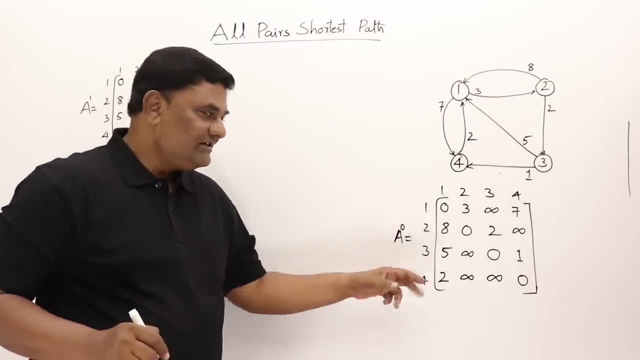 here. So those values are 0,, 3,, infinity and 7, and these are 8,, 0,, 3,, infinity and 7.. So 5 and 2.. So first row and first column already I have taken as it is. Then what about the? 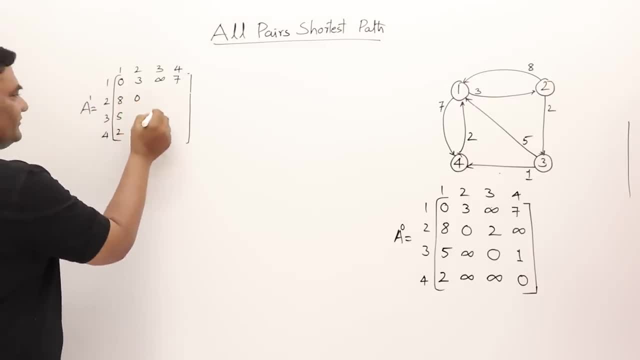 diagonals. There are no self loops, so I will fill those diagonals also. Now remaining values. I have to find out What are those. First, let us check this one, that is 2 to 3.. So how to get this value? How to check whether there is a shorter path via vertex 1 or not? So 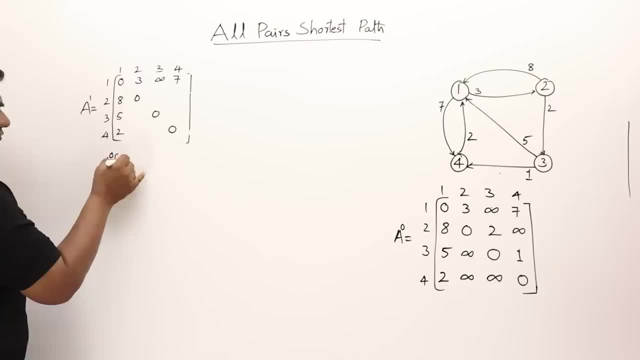 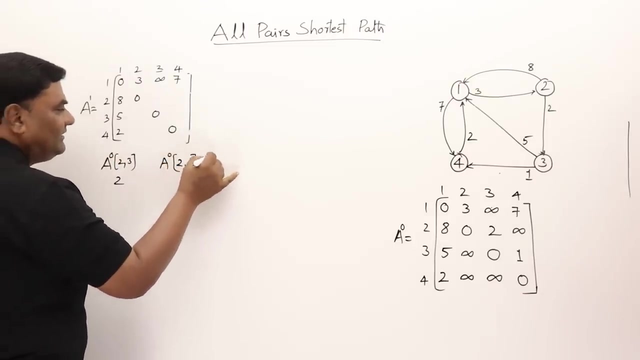 2 to 3, I will take A0 of 2 to 3.. So what is there in this matrix 2 to 3?? So 2 to 3 is a 2. And A0 of now. in between I should include vertex 1.. So 2 to 1 and 1. 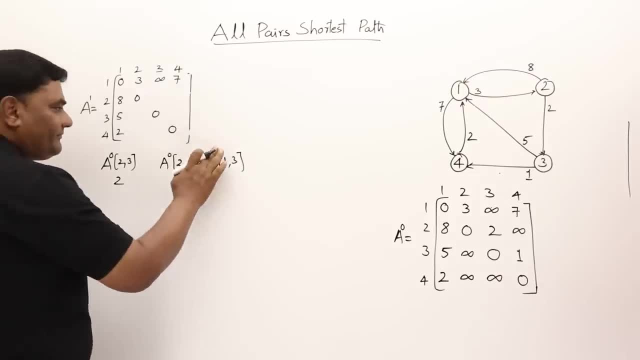 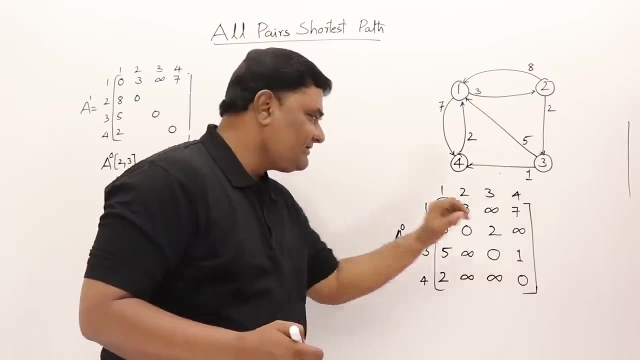 to 3 from those matrix. From that matrix 2 to 1 and 1 to 3.. 2 to 1 is how much? 8.. 1 to 3 is infinity. So this is 8 plus infinity. This is infinity, only This is less, So there. 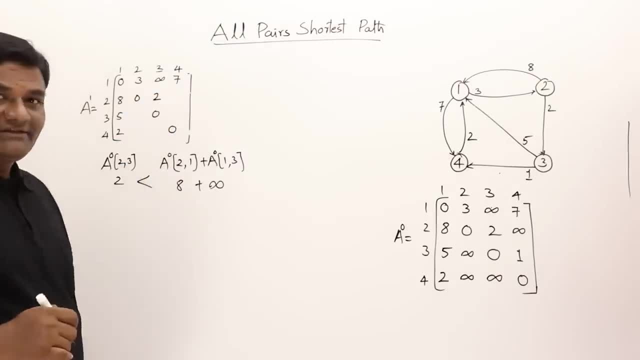 is no better path via vertex 1.. So let it be 2 only. Now I have to find out next one that is 2 to 4.. So A0 of 2 to 4.. What is the value there? 2 to 4? 2 to 4 is infinity. This is infinity. Now I should include: 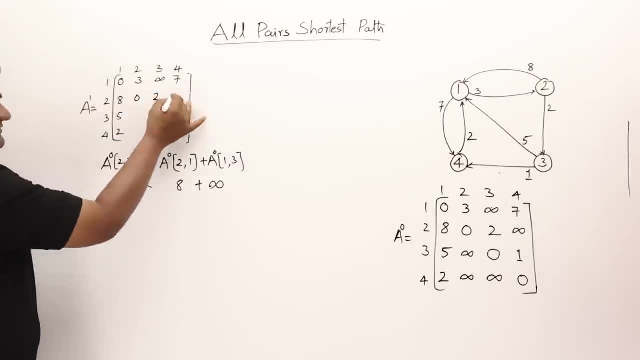 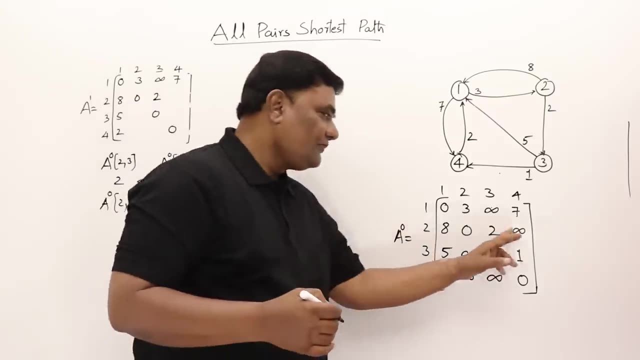 so let it be 2. only now i have to find out. next one that is 2 to 4. so a 0 of 2 to 4. what is the value there? 2 to 4. 2 to 4 is infinity. this is infinity. now i should include vertex 1 in between. 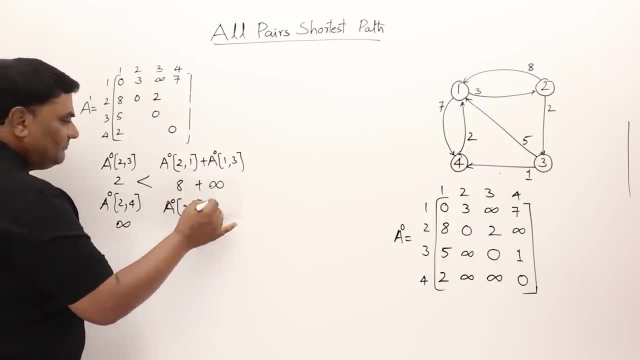 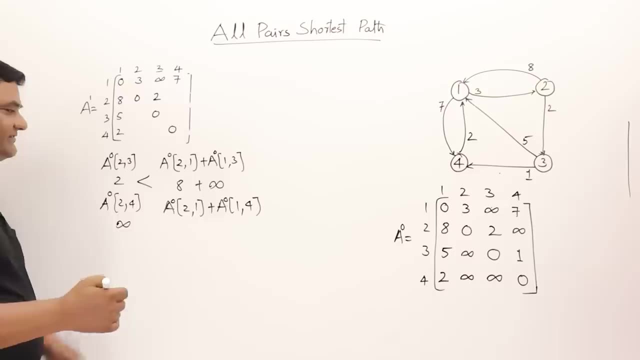 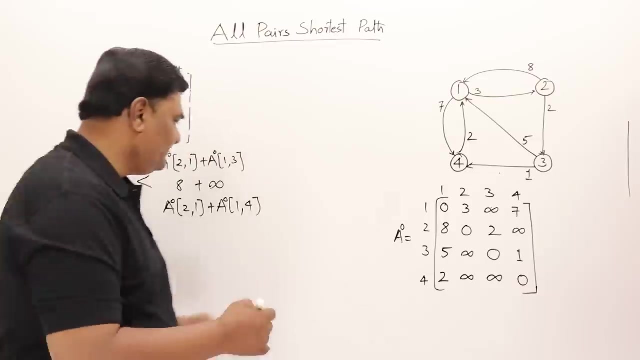 as an intermediate vertex, so a 0 of 2 to 1 plus a 0 of 1 to 4. so from that matrix find out 2 to 1 and 1 to 4. 2 to 1 is how much 8. then 1 to 4 is 7, 15. so this is 8 plus 7. this is 15. so this one is smaller than. 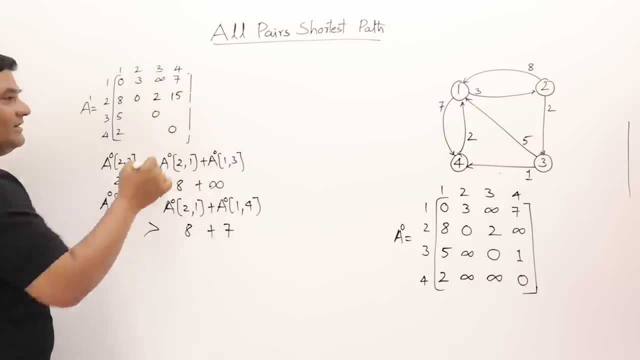 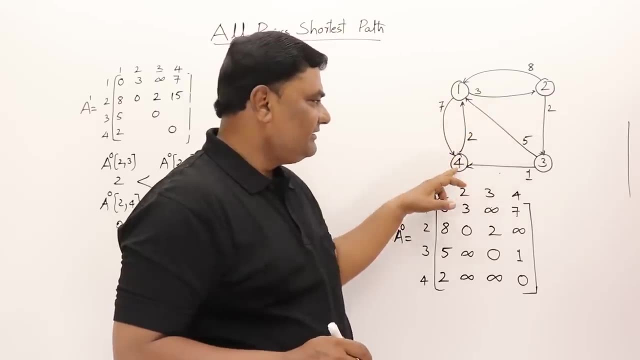 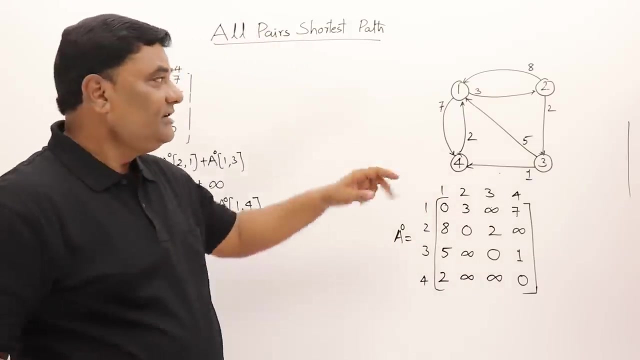 infinity. so update this path to 15. so this means that from 2 to 4, 2 to 4 there is no direct edge path, but 2 to 1, then 1 to 4, that is 8 plus 7, 15. there is a path going via vertex 1. that's what we. 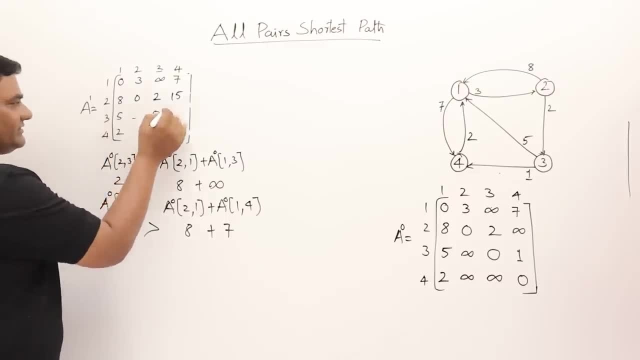 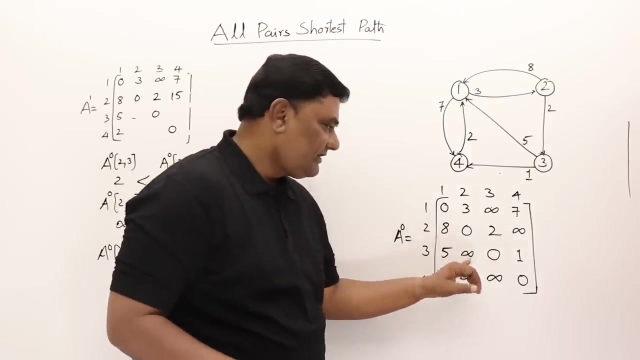 got the answer here. now i have to fill up these values right. so that is 3 to 2. so i'll find out a 0 of 3, 2. in between i should add 1, 3, 1, 1, 2. so 3 to 2 is how much. 3 to 2 is infinity: 3 1, 5. 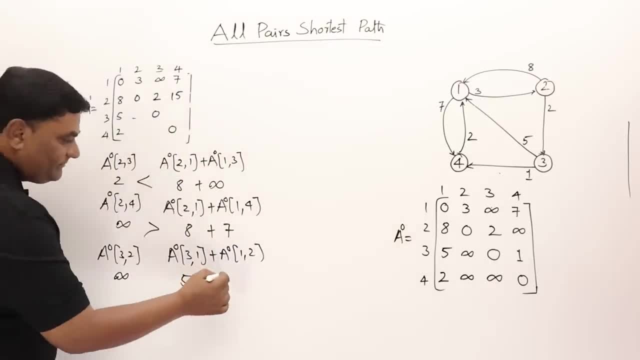 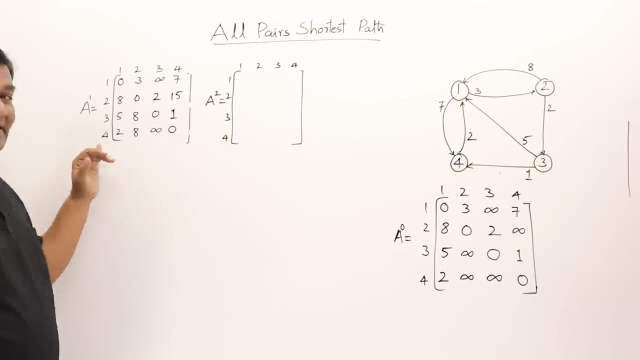 plus 1, 2 is a 3, so you can check there. here infinity is greater, so this value is smaller, that is 8. so we got a smaller value, 8. in the same way, i should fill up all these values. so i have prepared this matrix which is going via vertex 1. now i will prepare a matrix which is going via vertex 2. 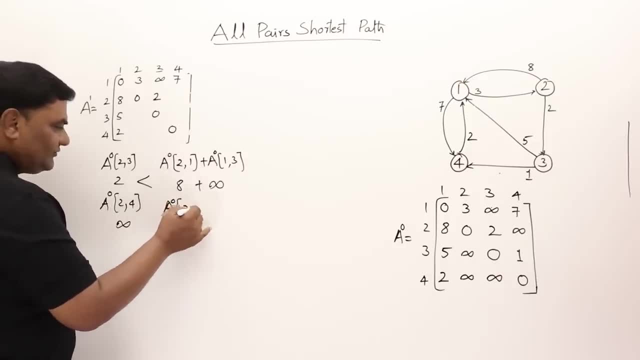 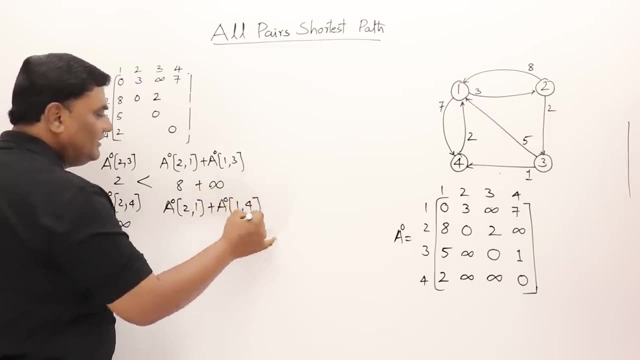 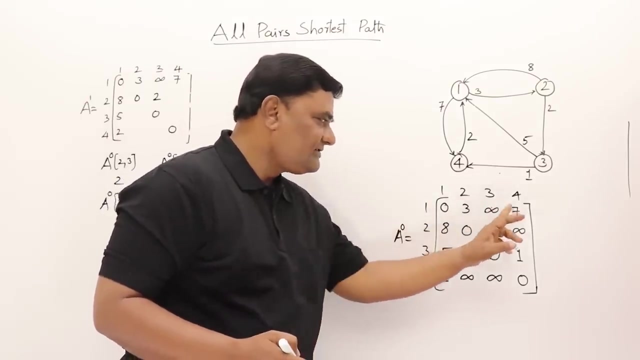 vertex 1 in between as an intermediate vertex. So A0 of 2 to 1 plus A0 of 1 to 4.. So from that matrix find out 2 to 1 and 1 to 4.. 2 to 1 is how much? 8. Then 1 to 4 is 7., 15. So this is 8 plus 7. This is 15.. So this. 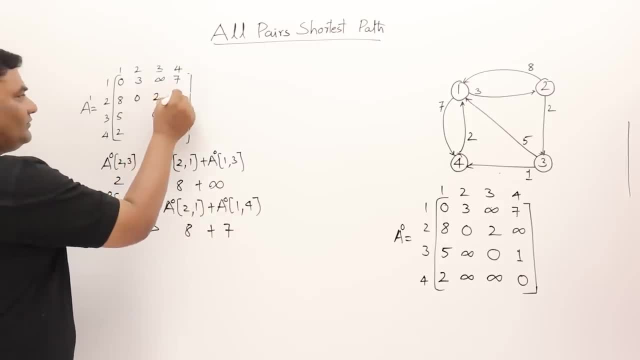 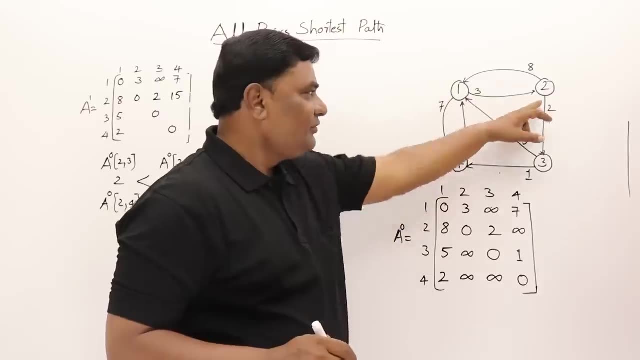 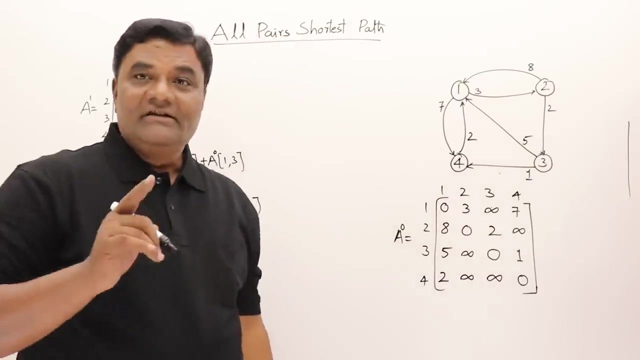 one is smaller than infinity, So update this path to 15.. So this means that from 2 to 4, 2 to 4 there is no direct edge path, But 2 to 1, then 1 to 4.. That is 8 plus 7. 15. There. is a path going via vertex 1.. That's what we got done. So this is the matrix 2 to 1.. 2 to 1 is how much 8.? Then 1 to 4 is 7. 15. So this is 8 plus 7.. This is 15.. So this. 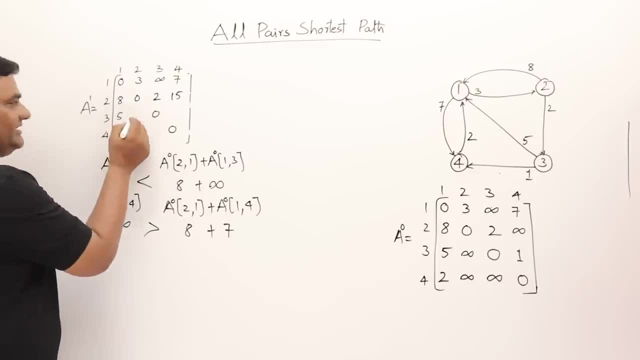 is 7.. There is no direct edge path. But 2 to 4 is 7.. So this is 8 plus 7. That is 8 to 4.. Now I have to fill up these values Right. So that is 3 to 2.. So I will find out. A0. 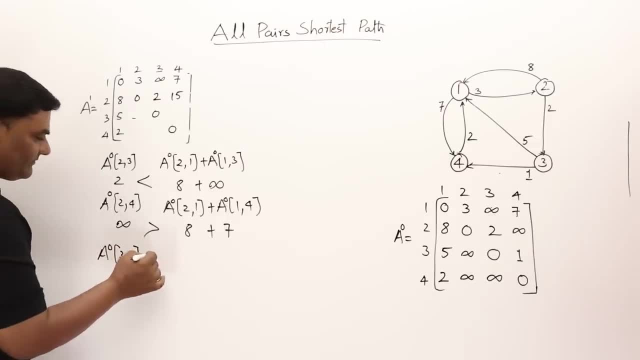 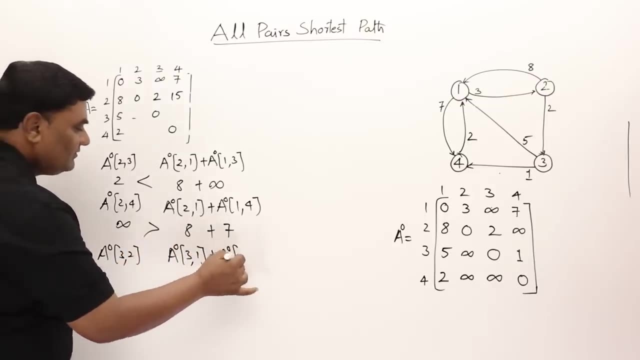 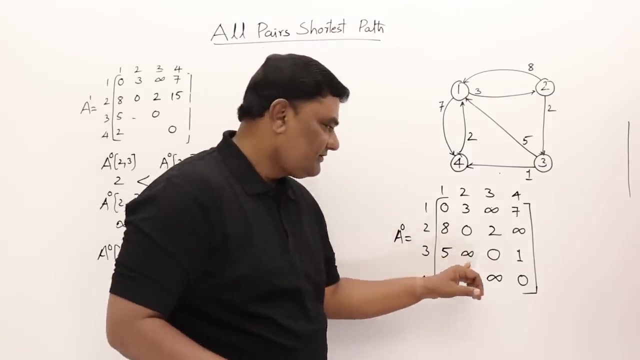 of 3 to…in between I should add 1, 3, 1, 1, 2.. So 3 to 2 is how much? 3 to 2 is infinity: 3,1.. 0 to 1.. 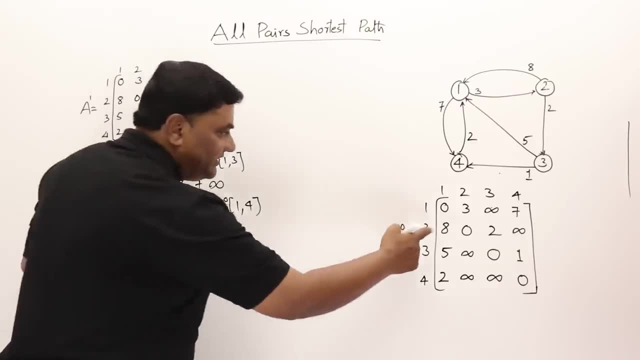 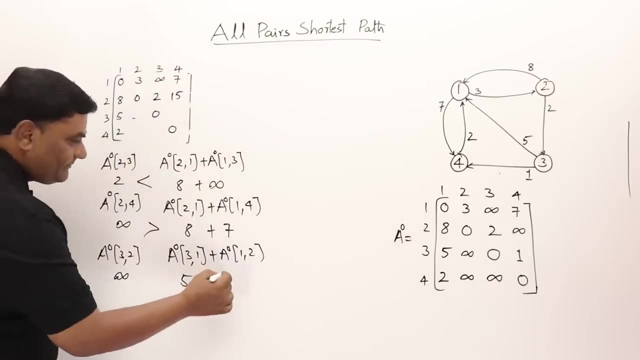 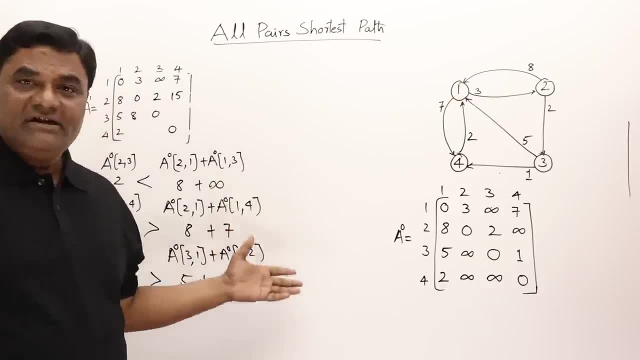 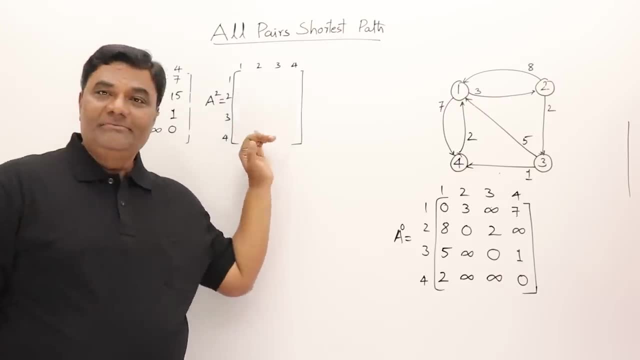 So we got a smaller value, 8. in the same way, I should fill up all these values. So I have prepared this matrix which is going via vertex 1. now I will prepare a matrix which is going via vertex 2, so I should generate this matrix from this matrix. 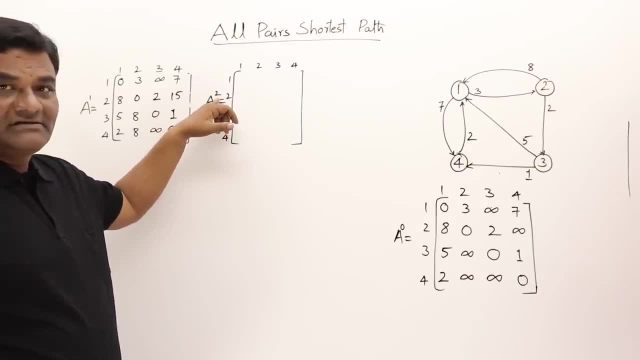 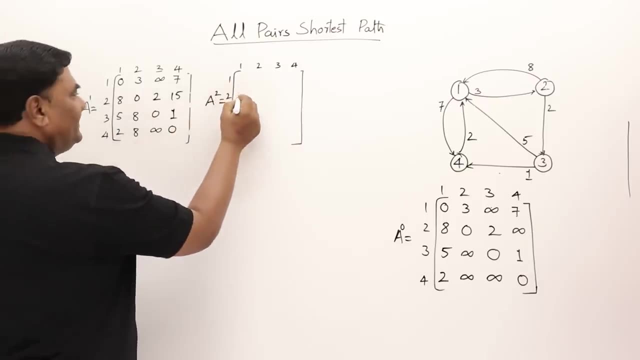 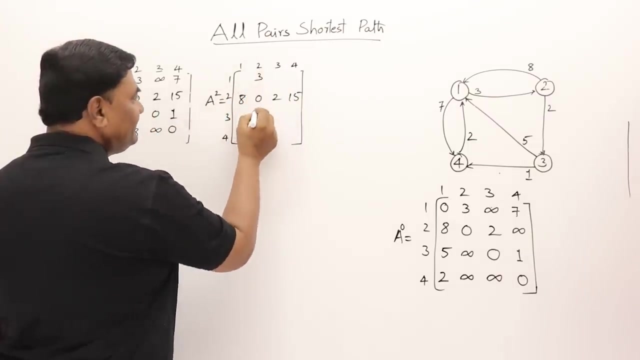 So when I am taking a second matrix to as a intermediate vertex, then Second row and second column remains as it is. so I will take this second row, second column as it is 8, 0, 2 and 15, second column is 3 0, 8, 8, 3 0, 8, 8 and the diagonals remains. 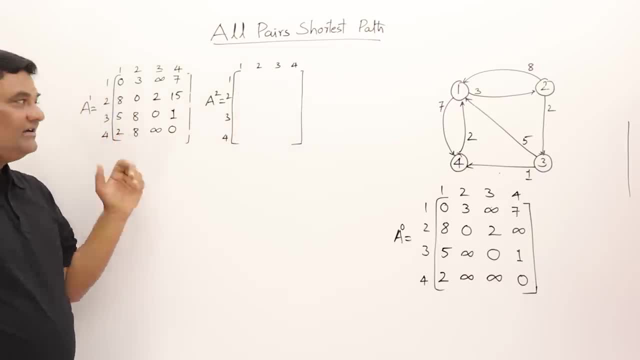 so i should generate this matrix from this matrix. so when i am taking a second matrix, 2 is the intermediate vertex, then second row and second column remains as it is. so i will take the second row, second column as it is 8, 0, 2 and 15. the second column is 3088- 3088. 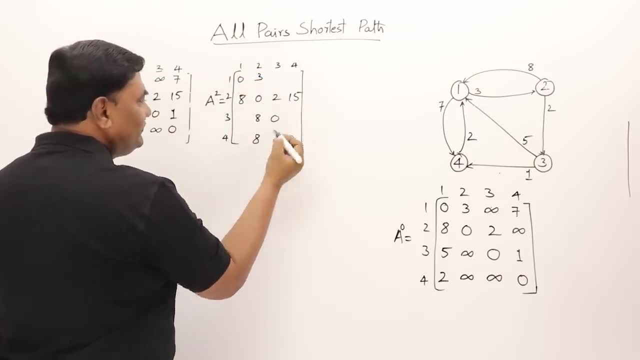 and the diagonal is remain 0. only now i have to find out few values here. what are those? first one is 123. let me find out from this matrix: A1 of 1.5-2-3 is cum句 A1 of 1 comma 3. 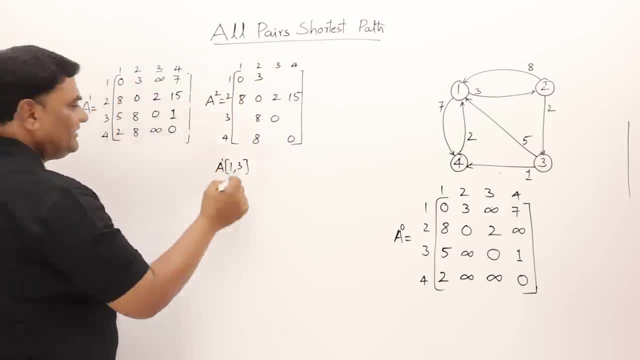 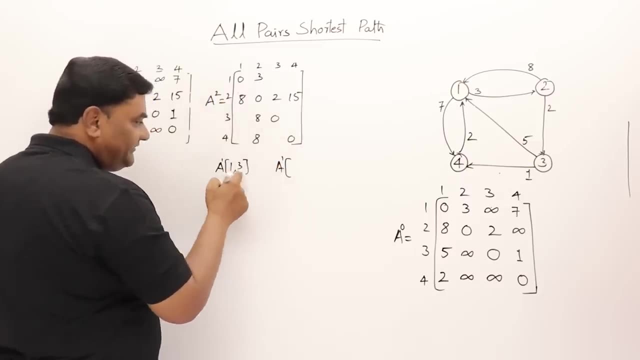 A1 of 1 comma 3. Here 1 comma 3 is what Infinity? Then in between I should include vertex 2, So A1 of in between 1 to 3, So 1 to 2 plus A1 of 2 to 3. 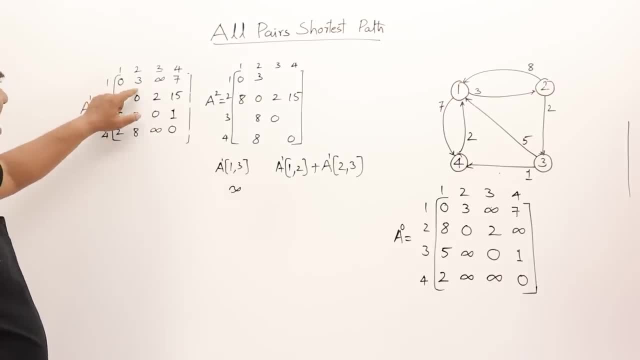 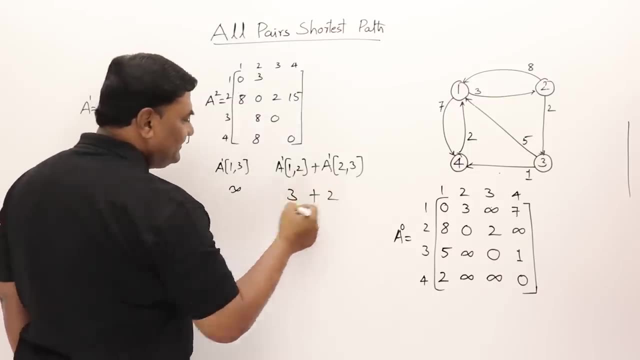 Check this one: 1 to 2 is 3 and 2 to 3 is 2, So this is 3 plus 2, that is 5 and this is smaller. Update this Now. this was infinity. Now we got a path via vertex 2. 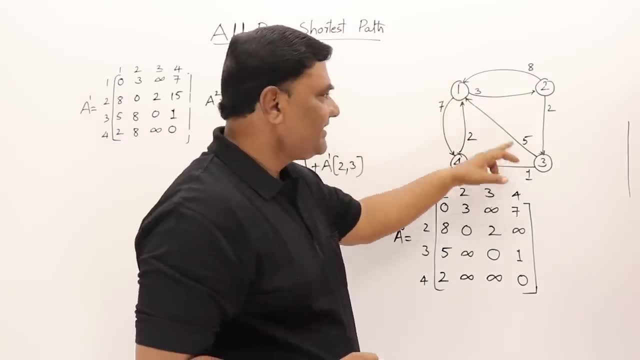 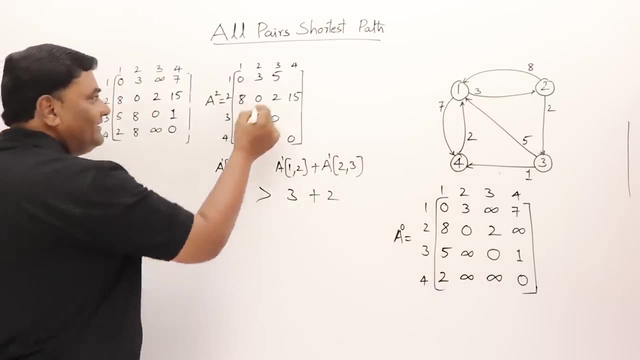 in between 1 and 3. 1 to 3. There is a path going to 2, then 3, So 3 plus 2 is 5. We got a path here, So that's it. Now. I should give this value 1 to 4. 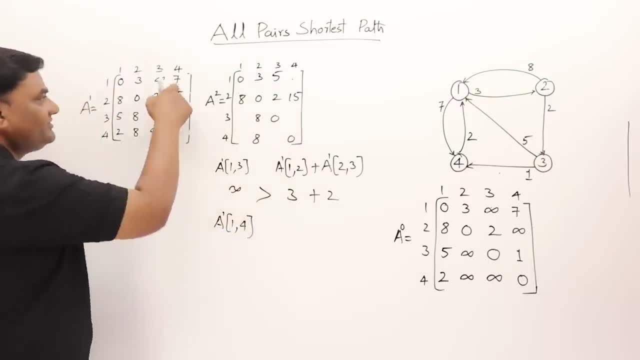 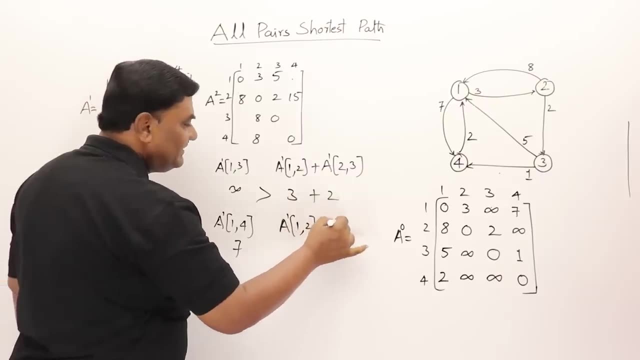 So A1 of 1 comma 4 is how much here 7, Then in between I should introduce vertex 2, So 1 to 2, plus A1 of 3, 2 to 4, So 1 to 2 is how much. 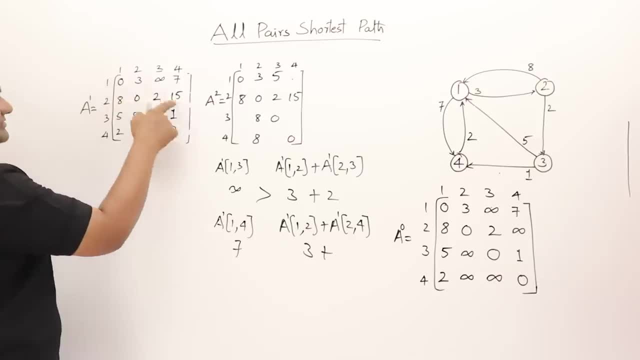 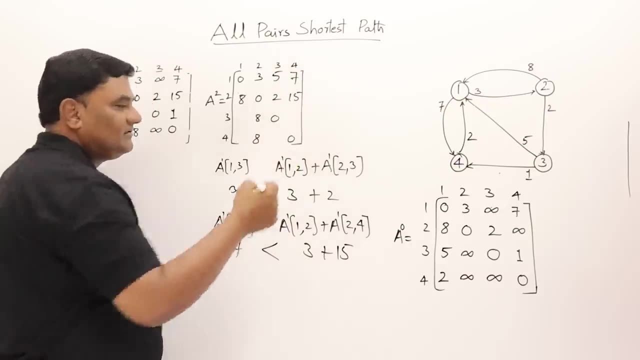 3 plus 2 to 4 is how much? 15. So this is 18, But this 7, which is already there, which is better. So take this 7 Now. in the same way, I should fill up all these values Already. I have prepared this. 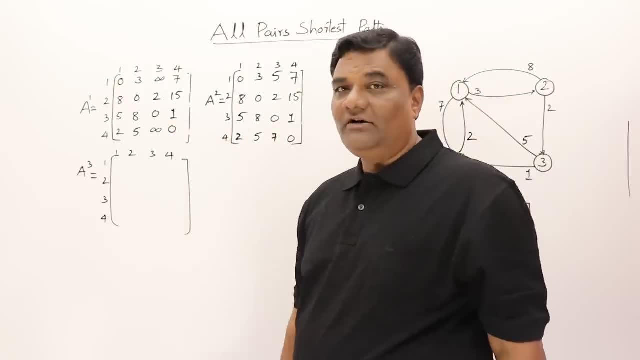 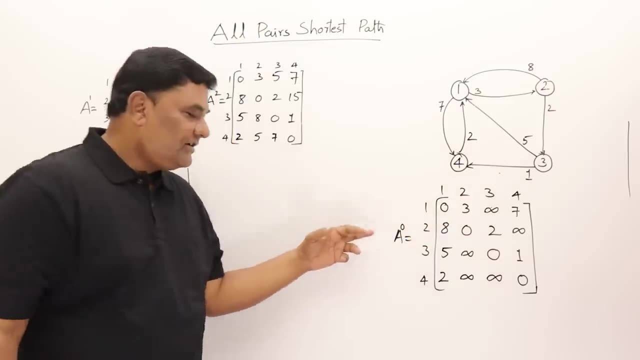 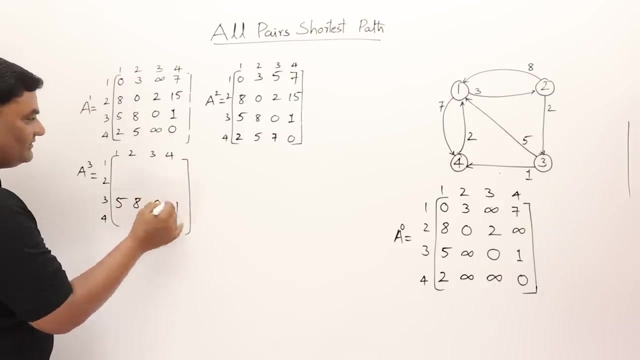 Vertex 2 as an intermediate vertex. Now I have to find out vertex 3 as an intermediate vertex and generate the matrix. When I say 3 as an intermediate vertex, Then the 3rd row and 3rd column remains as it is. So this is 5, 8, 0, 1. 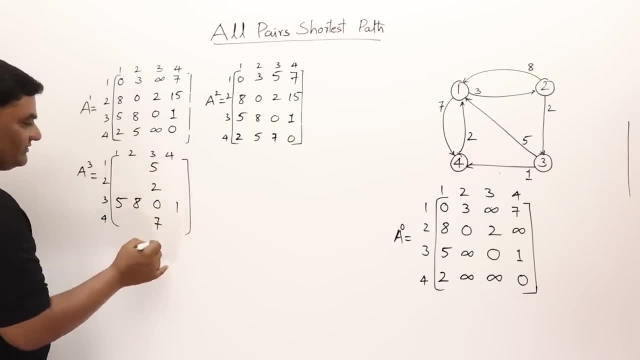 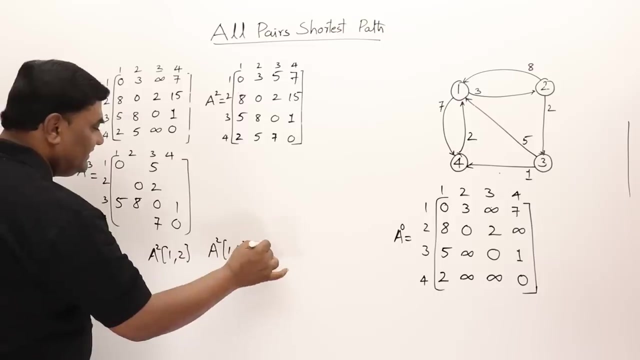 And this is 5,, 2,, 0,, 7, And the diagonals are 0, A2 of 1 comma 2, And in between I should take intermediate vertex as 3, Then A2 of 3 comma 2, Then A2 of 3 comma 2. 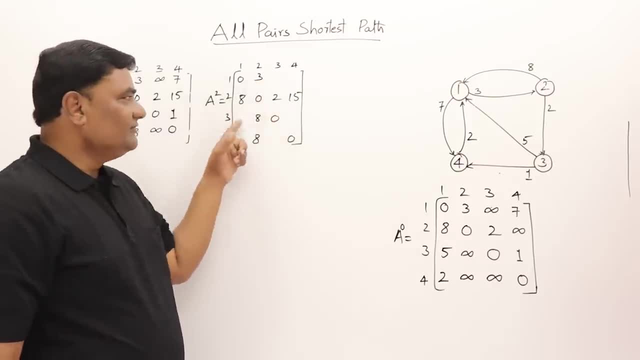 0. only Now I have to find out few values here. What are those? first one is 1, 2, 3?. Let me find out From this matrix: a 1 of 1 comma 3, a 1 of 1 comma 3. here 1 comma 3 is what infinity. 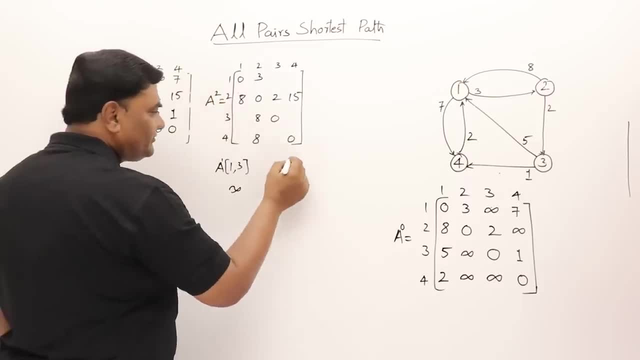 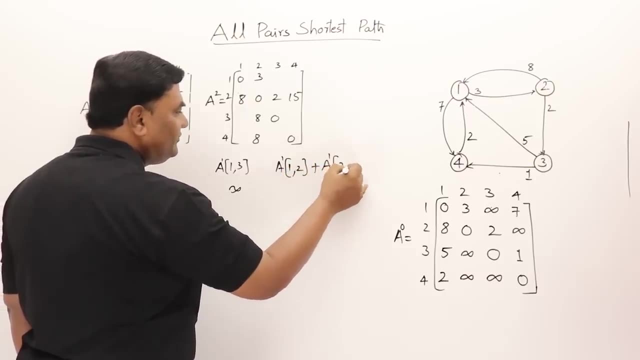 Then in between I should include vertex 2, so a 1 of in between 1, 2, 3, so 1, 2, 2 plus a 1 of 2, 2, 3. check this one: 1, 2, 2 is 2, 3 and. 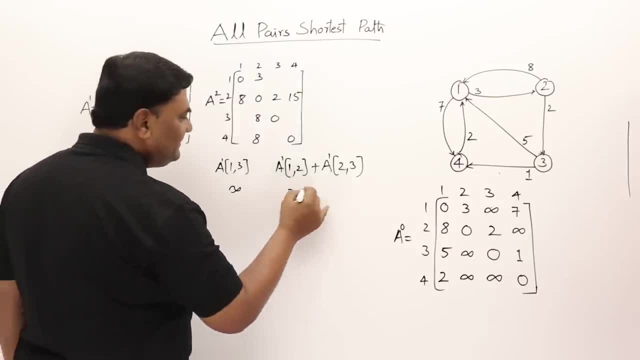 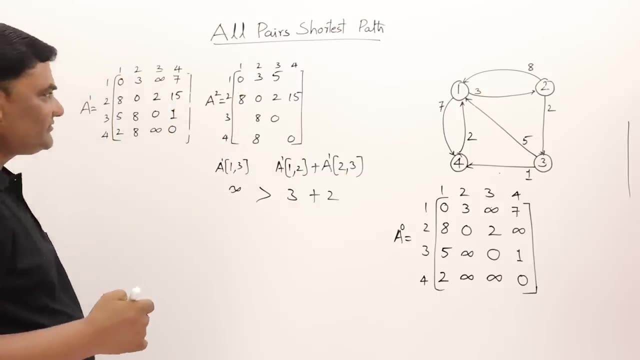 2, 2. 3 is 2, so this is 3 plus 2, that is 5 and this is smaller. update this now. this was infinity. now we got a path via vertex 2 in between 1 and 3. 1, 2, 3. 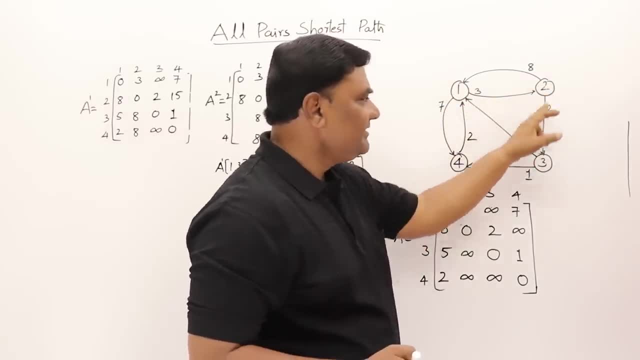 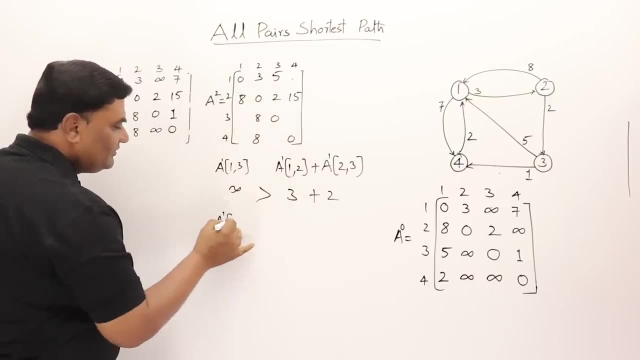 There is a path going to 2, then 3, so 3 plus 2, 5. we got a path here, So that's it. now I should get this value 1 to 4, so a 1 of 1 comma 4 is how much here? 7. 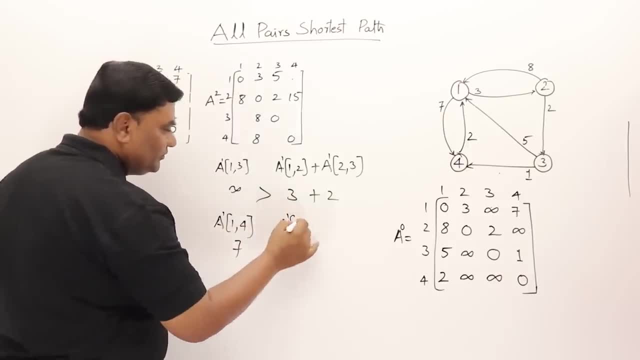 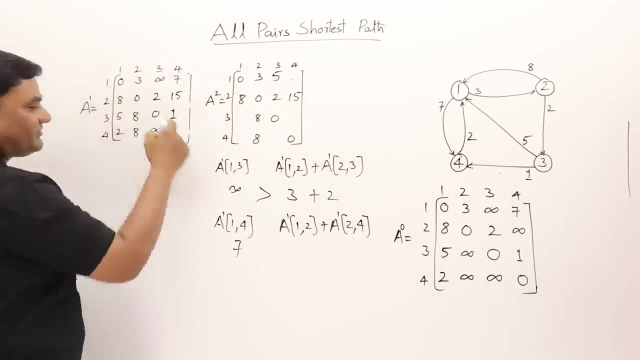 then in between I should introduce vertex 2, so 1 to 2, plus a 1 of 2 to 4. So 1 to 2 is how much 3?? plus 2 to 4 is how much 15, so this 18, but this 7, which is already there, which is better, so take this 7. 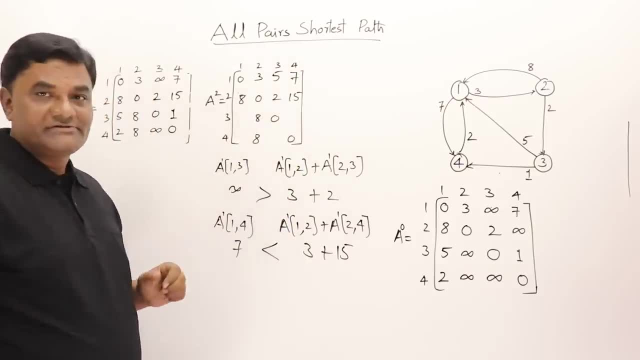 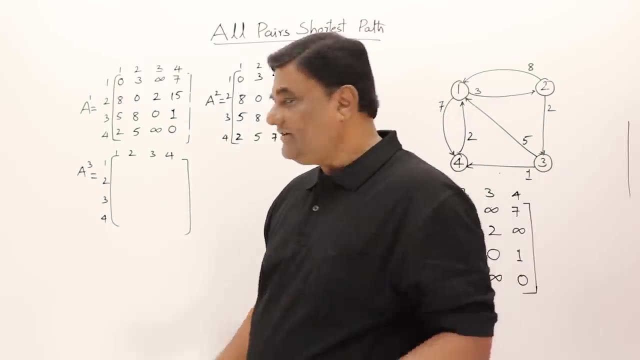 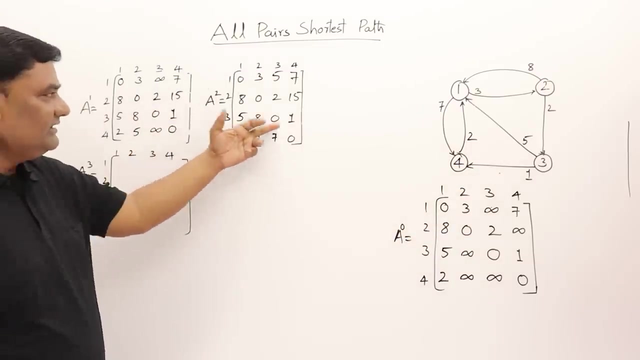 now in the same way. I should fill up all these values already. you have prepared this: what extrude as a intermediate vertex. now I have to find out what x3 as intermediate vertex and generate the Metrix. when I say 3 as the intermediate vertex, then the third row and third column remains as it is. So this is 5, 8, 0, 1. 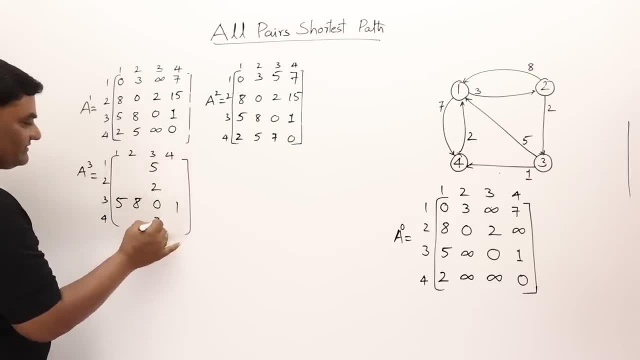 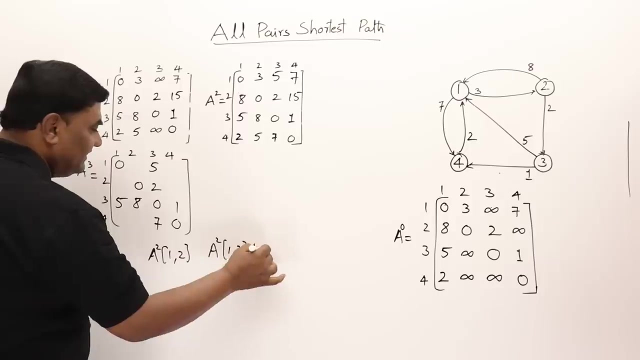 and this is 5,, 2,, 0,, 7 and the diagonals are 0.. a2 of 1 comma 2 and in between I should take intermediate vertex as 3, then a2 of 3 comma 2.. So 1 to 2 is there, so in between, 3 is there and 3. 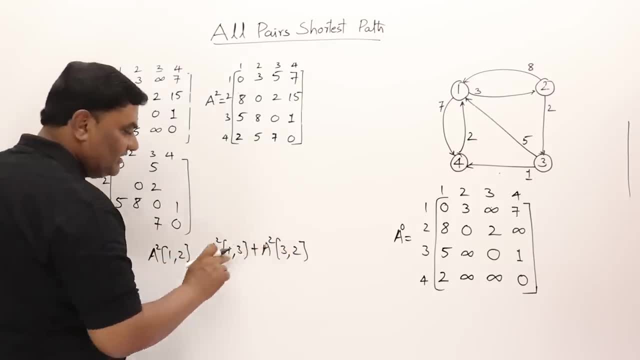 So 1 to 2 is there. So in between 3 is there and 3, 1 to 3 and 3 to 2. So out of this which one is smaller? 1 to 2. 1 to 2 is how much. 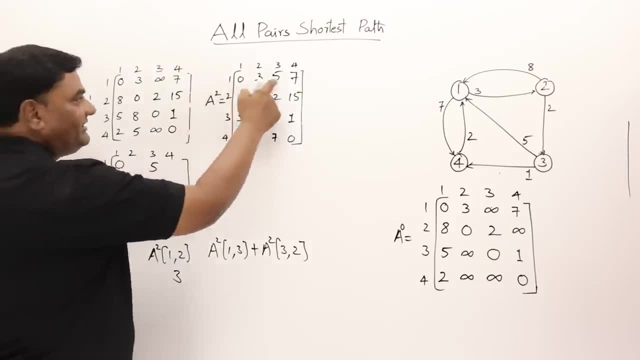 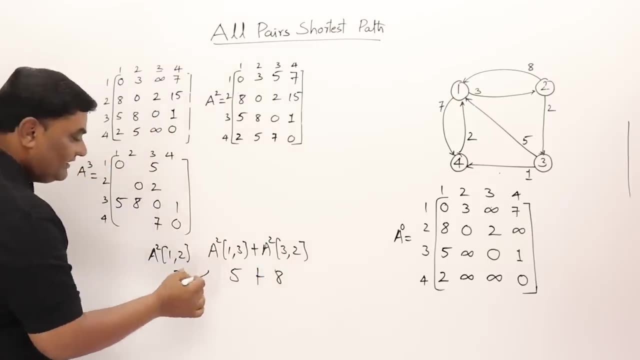 3 there And 1 to 3 is how much. 1 to 3 is 5 Plus 3 to 2. 3 to 2 is 8. 5 plus 8 is 13. This 3 itself is smaller, So take 3 only. 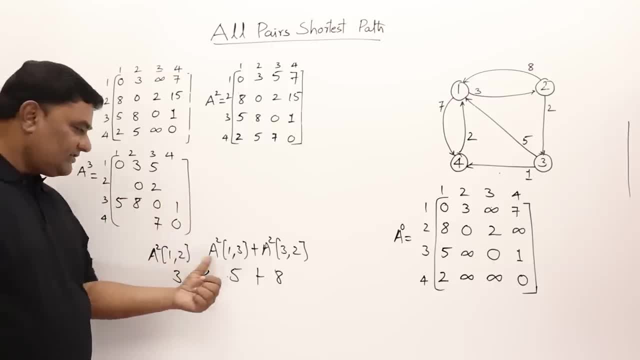 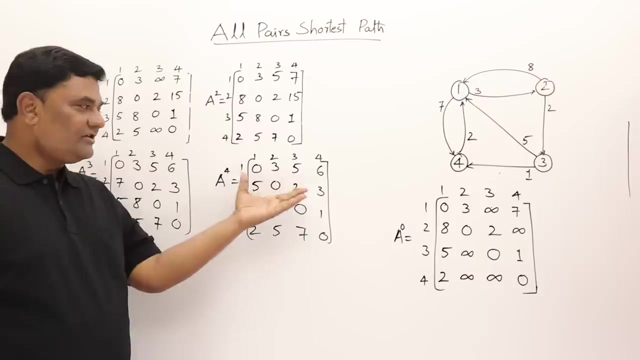 In the same way, I can find out all these values by taking 3 as intermediate vertex. Now I hope you have understood How I am getting the values, So I will prepare all the matrices. So here are the 4 matrices. Finally, the 4th vertex, When I considered I got a shortest path between all pair of vertices. 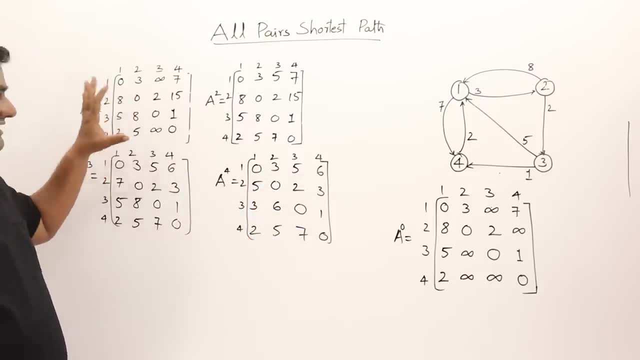 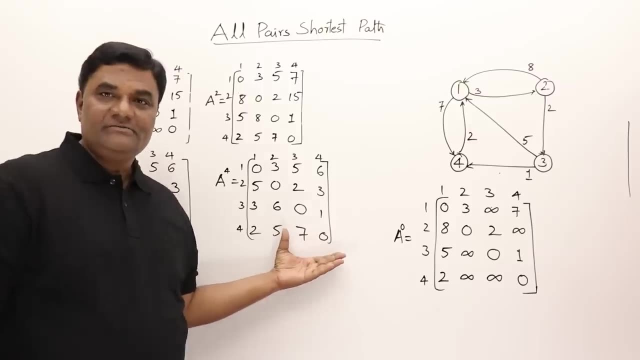 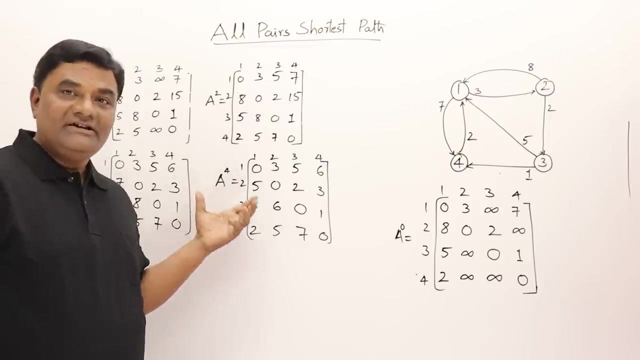 So we have taken sequence of decision. in each stage. We were getting a matrix here, The table is like a matrix here And finally, these are the shortest paths Between every pair of vertex. What was the formula I was using? I will prepare the formula Getting the value of any matrix. 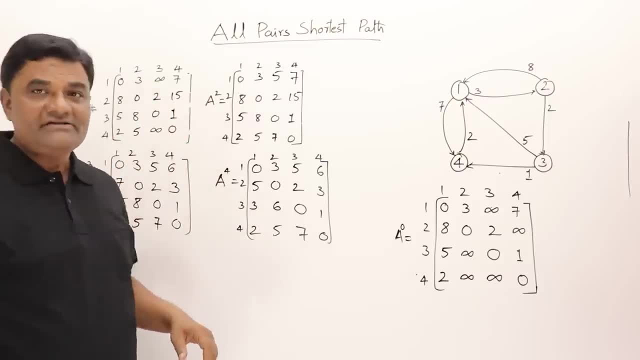 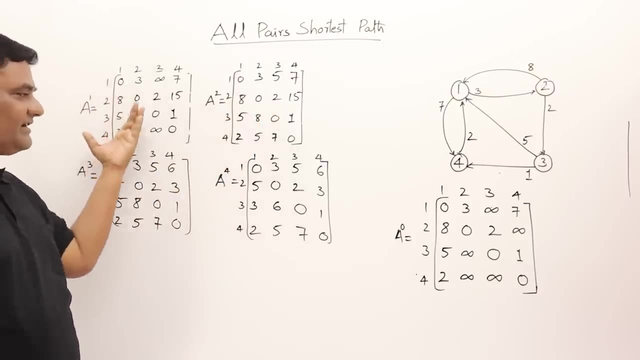 Let us say 4 is the intermediate vertex Or 2 is the intermediate vertex. So when I was selecting one of the vertex as the intermediate vertex, Then how I was getting the values here, I was getting from the previous matrix For 4, I was getting from 3. 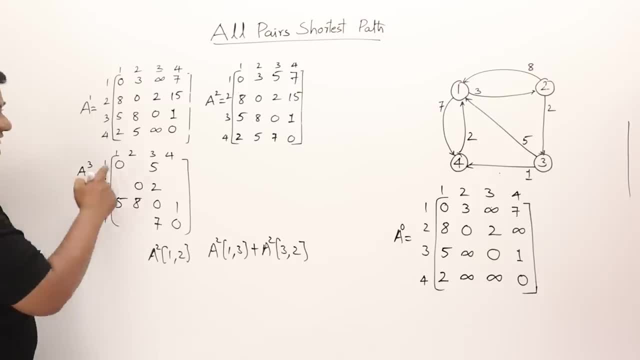 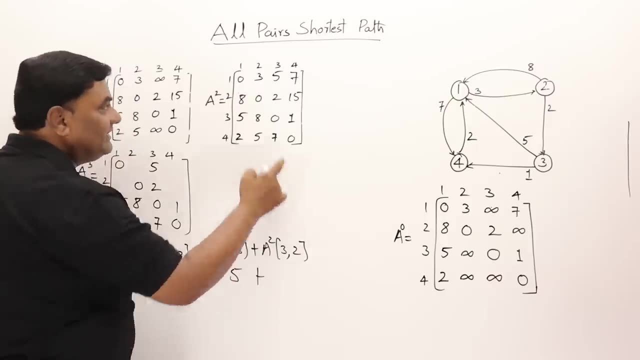 1 to 3 and 3 to 2.. So out of this, which one is smaller, 1 to 2?? 1 to 2 is how much 3 there, and 1 to 3 is how much. 1 to 3 is 5 plus 3 to 2.. 3 to 2 is 8.. 5 plus 8, 13. This 3 itself is 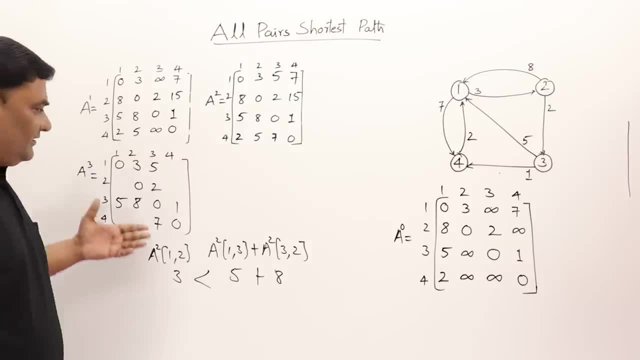 smaller. so take 3 only. In the same way, I can find out all these values by taking 3 as intermediate vertex. Now I hope you have understood how I am getting the values, So I will prepare all the matrices. So here are the four matrices. Finally, the fourth vertex, when I considered I got a shortest path between all. 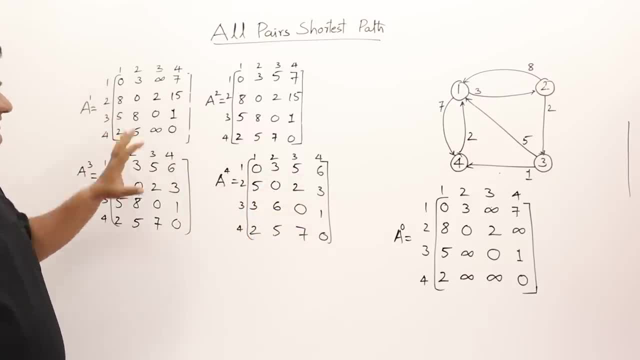 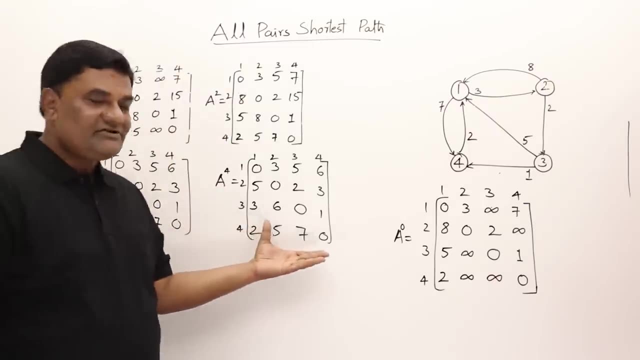 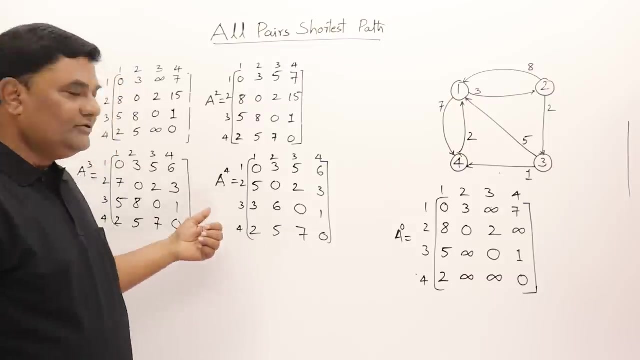 pair of vertices. So we have taken sequence of decision in each stage. we were getting a matrix here, The table is like a matrix here and finally, these are the shortest. What was the formula I was using? I will prepare the formula For getting the value of any. 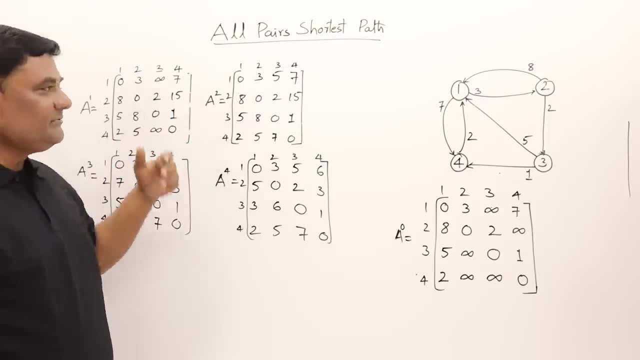 matrix. let us say 4 is the intermediate vertex or 2 is the intermediate vertex. So when I was selecting one of the vertex as the intermediate vertex, then how I was getting the values here, I was getting from the previous matrix. For 4 I was getting from 3,. for 3, I got from 2.. 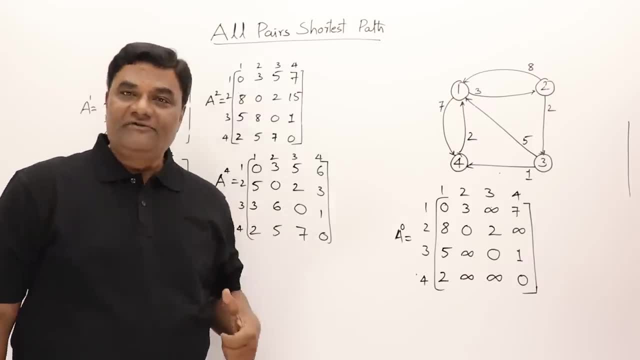 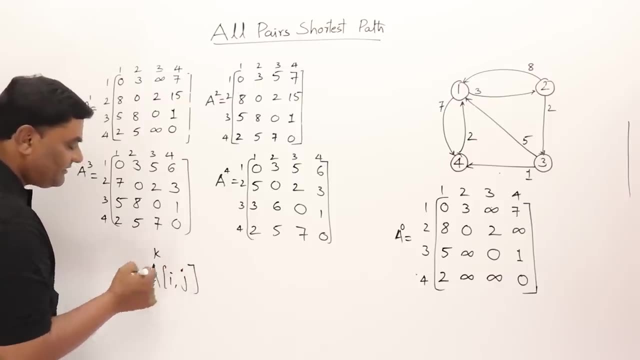 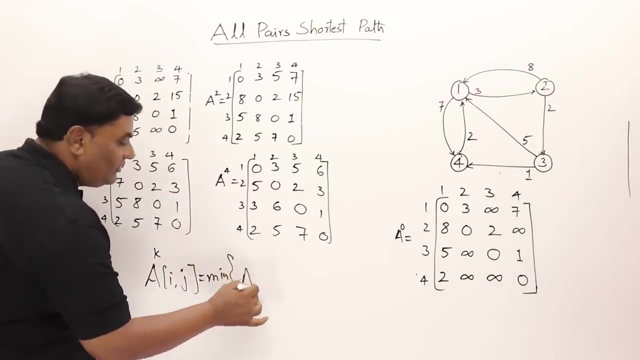 For 3, I got from 2, So how the formula can be framed. So now I will show you the formula For getting A of of any intermediate vertex, Any value from any intermediate vertex. I am taking minimum of A of from which matrix? Previous matrix. 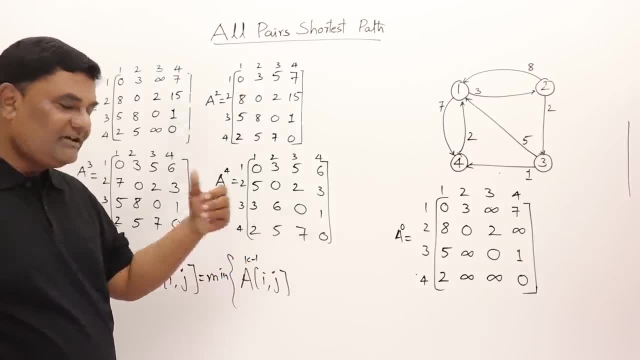 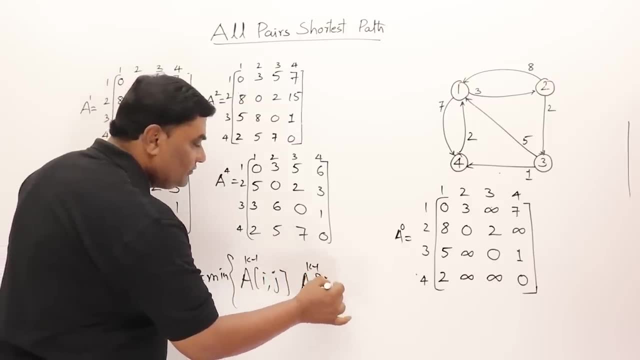 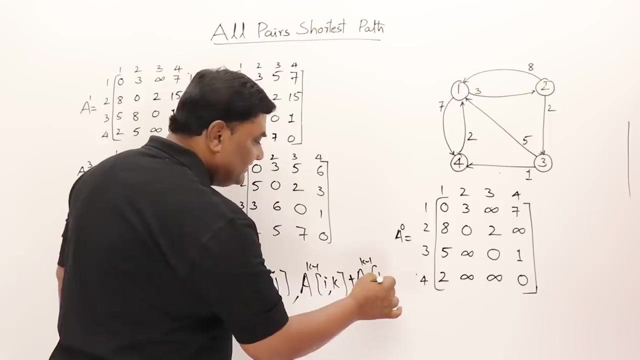 That is K-1. If I am generating K at the matrix, Then I was taking the value from K-1, Either this Or A of I to K Vertex, K Intermediate vertex, as K Plus A of Then K to J. So here you can see that K is introduced in between. 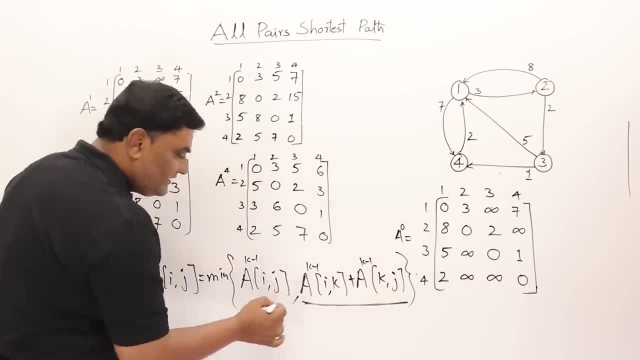 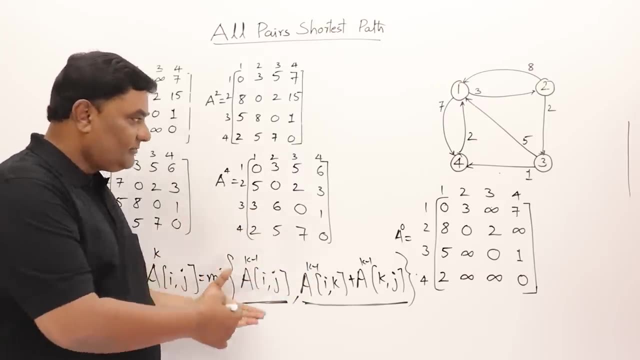 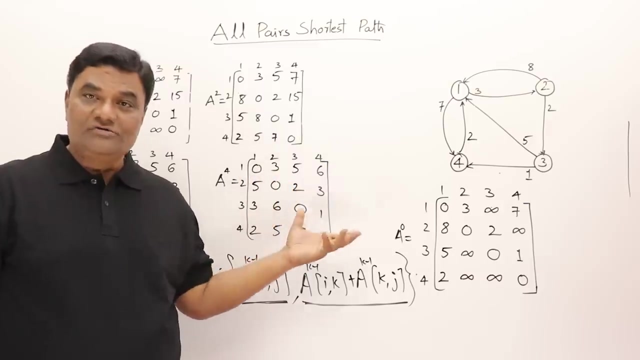 And addition is done. So either this one is smaller Or this one is smaller Out of this. whichever one is smaller, I was getting that one And I was following the same formula For generating all the matrices. I have shown only few terms. That is sufficient for understanding the approach. 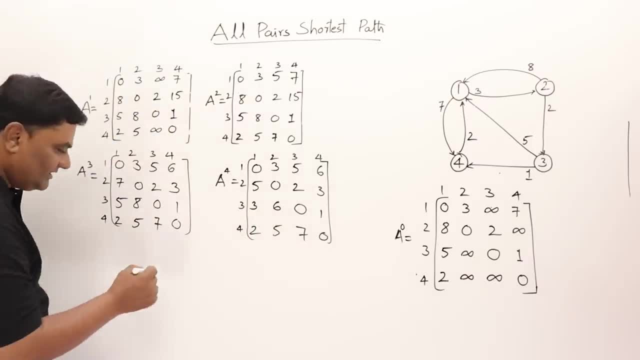 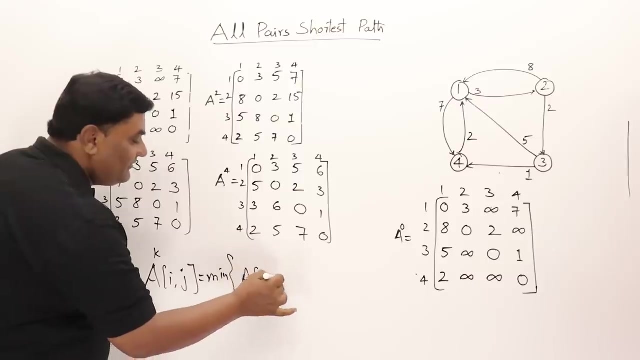 So how the formula can be framed. So now I will show you the formula For getting a of i comma j, For getting a of any intermediate vertex, any value from any intermediate vertex. I was taking minimum of a of i comma j from which matrix, Previous matrix, that is k minus 1.. If I am 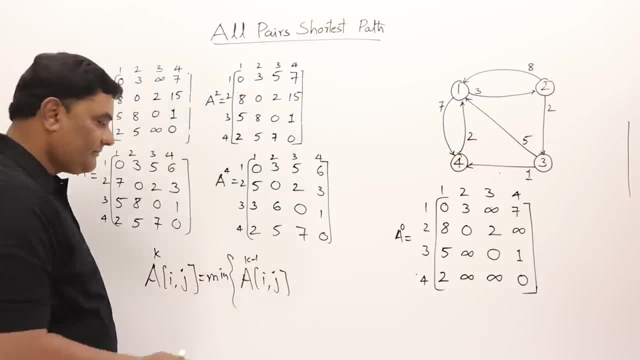 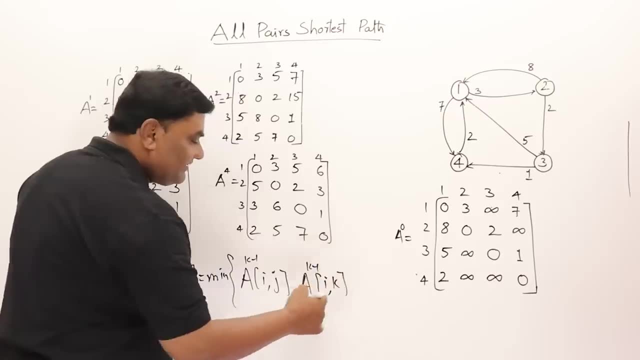 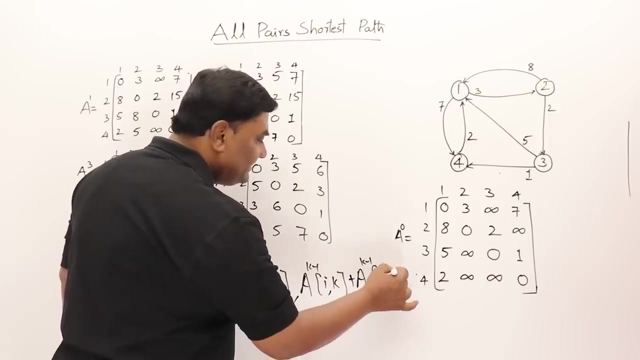 generating k at the matrix, then I was taking value from k minus 1.. Either this or a of k minus 1 i to k vertex, k intermediate vertex as k plus a of k minus 1 i to k vertex, k intermediate vertex, then k to j. So here you can see that k is introduced in between and addition is done. 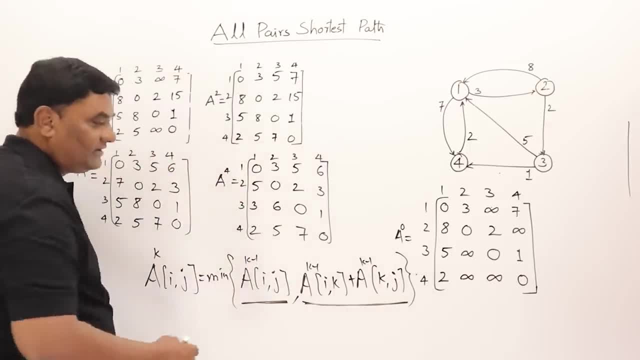 So either this one is smaller or this one is smaller Out of this. whichever one is smaller, I was getting that one and I was following the same formula for generating all the matrices. I have shown only few terms. that is sufficient for understanding the approach and how the 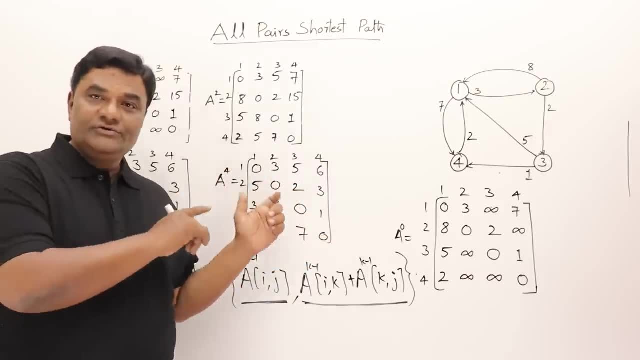 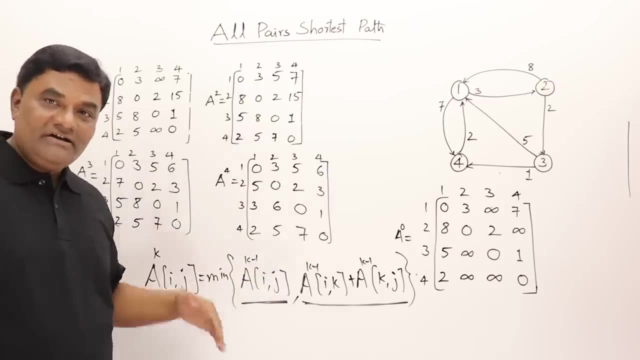 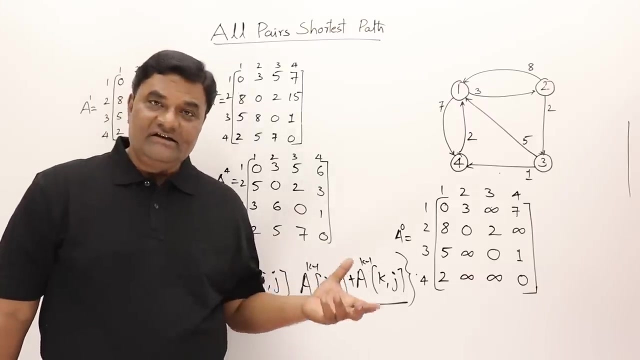 And how the formula is used. See, I have first shown you the working, Then I have generated the formula. Instead of following the formula, I have deduced the formula. That is it. Now let me show you How the code looks like, If I am writing the code. Now let us look at the code. 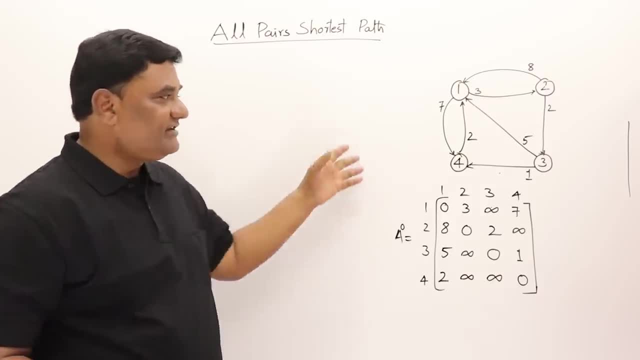 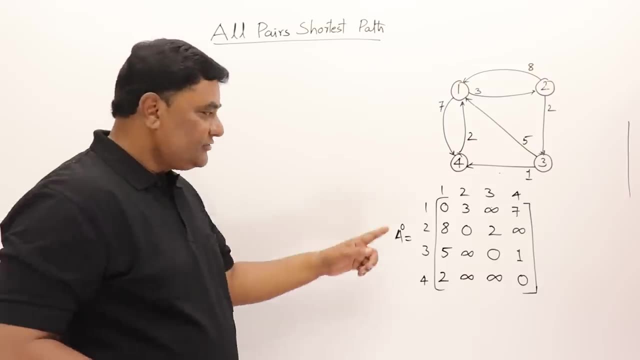 Every time I was generating the matrix. So how many such matrices I have generated? 4 such matrices I have generated. Now, for generating a matrix, What I am supposed to do- I should generate each and every term. So, total, how many terms are there? See, the number of vertices are 4. 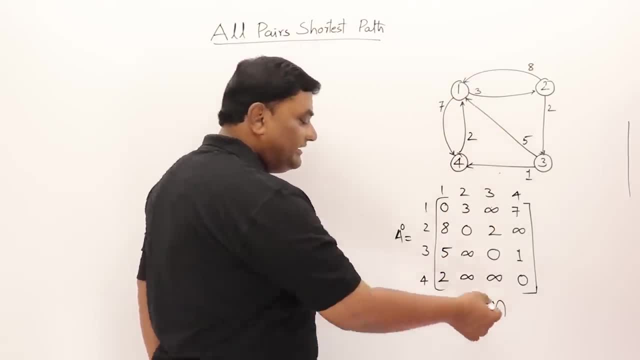 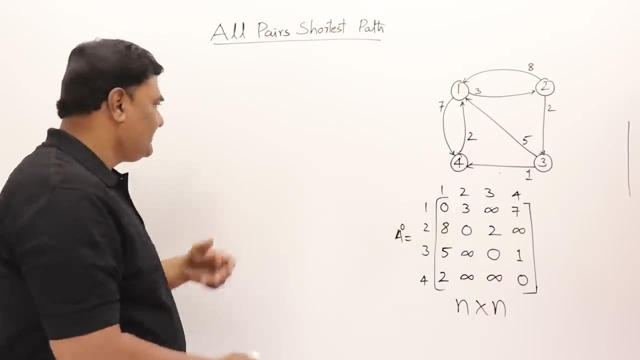 So let us say N vertices. So the number of elements are N, x, N. This is a square matrix. Now for getting all the elements of a square matrix, I should have 2 for loops. So I will take 2 for loops, For i assigns 1, i less than or equal to N. 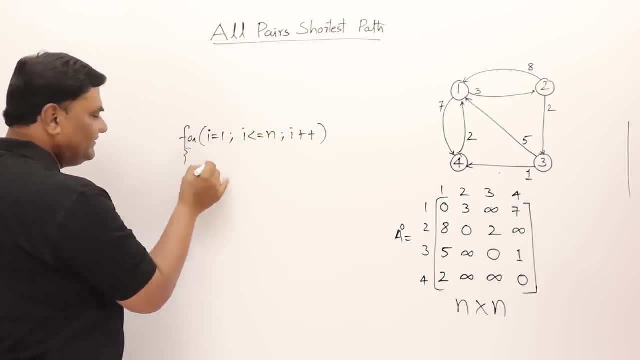 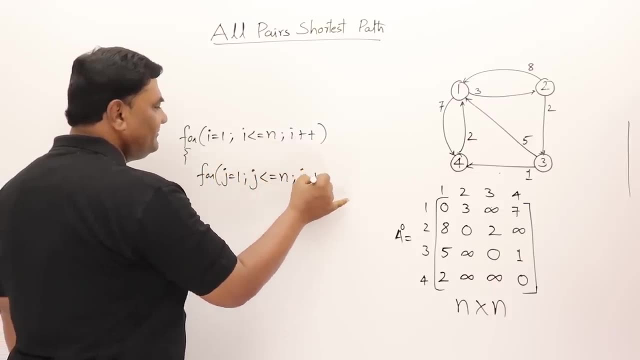 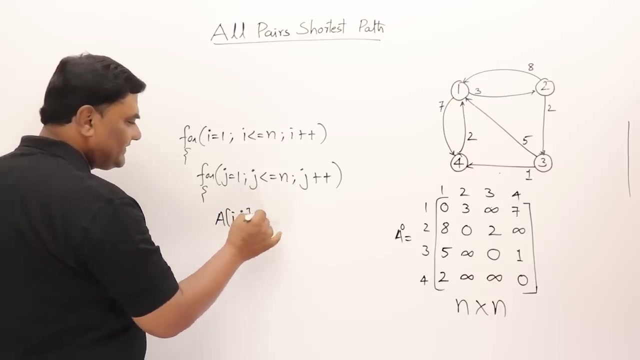 i++ And For j assigns 1. j is less than or equal to N j++, And I should get the terms of i comma j As minimum of a of i comma j. That is existing matrix As it is going to be a single instance of 2D array. 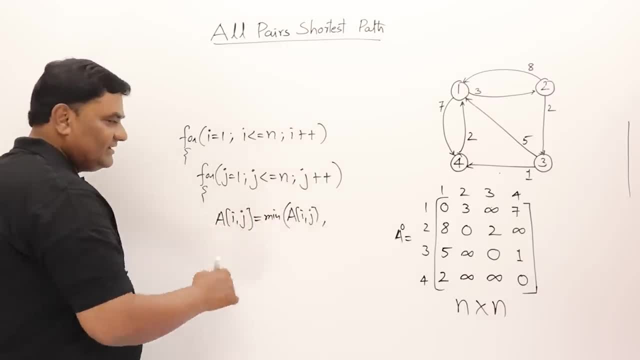 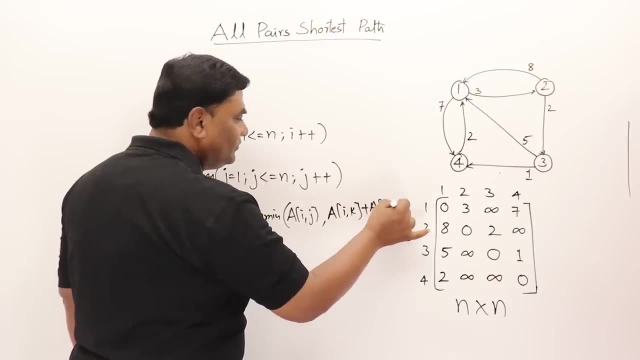 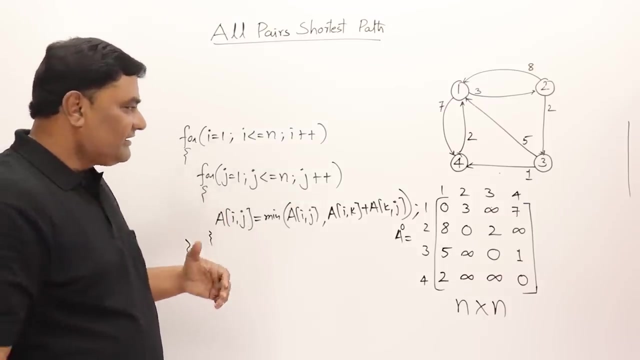 In the single instance only, I will be updating the values, So that is why this is same thing. Then a of i to k Plus a of k to j. Out of this I should select any one of them, Whichever is minimum. So what is k here? k will be changing the intermediate matrices. 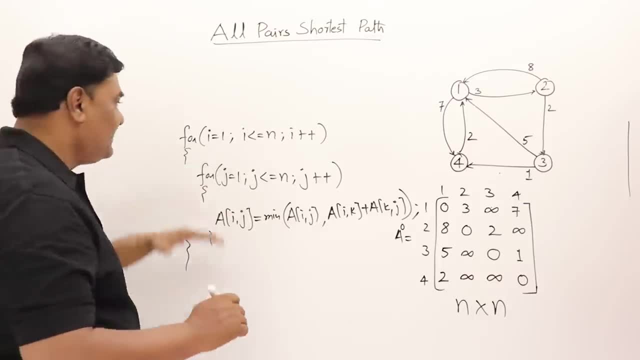 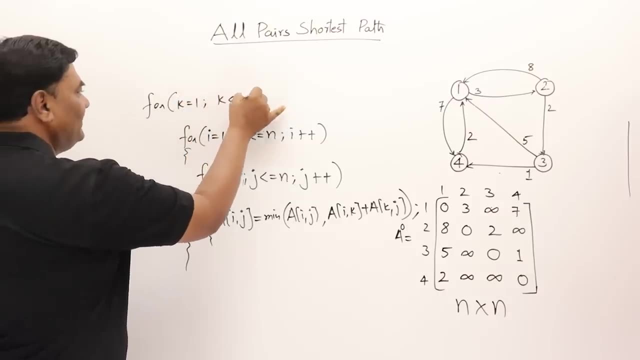 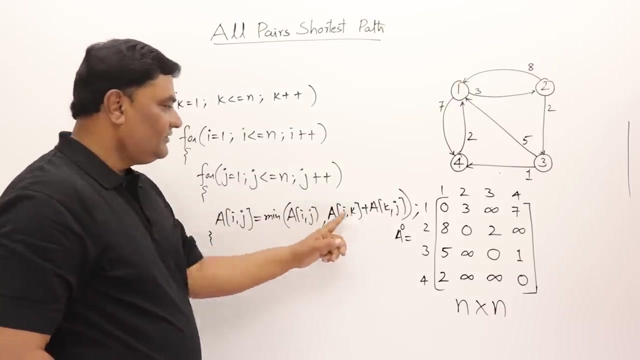 So this whole thing Will generate just one matrix And I have to generate all the matrices. So for k assign 1. k is less than or equal to N, k++. Now, first time k will be 1, So the intermediate vertex will be 1 all the time. 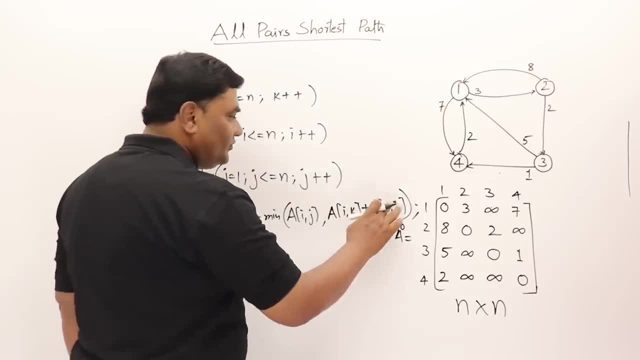 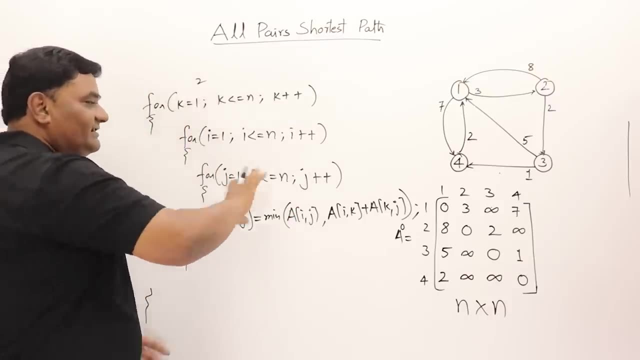 Then k is 2, So the intermediate vertex will be 2 all the time, So k will take this value. So when k is 1, then the matrix is 0, Then k is 2, Then the second matrix is generated. So this is for generating a matrix. 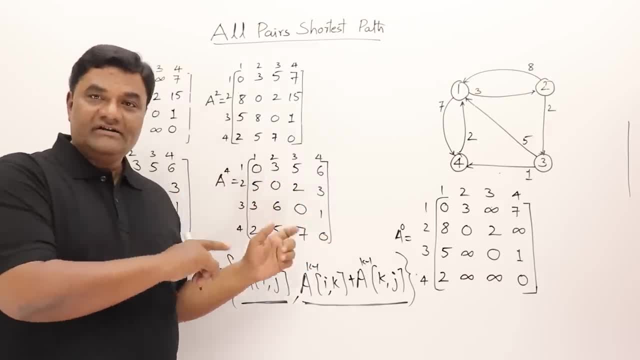 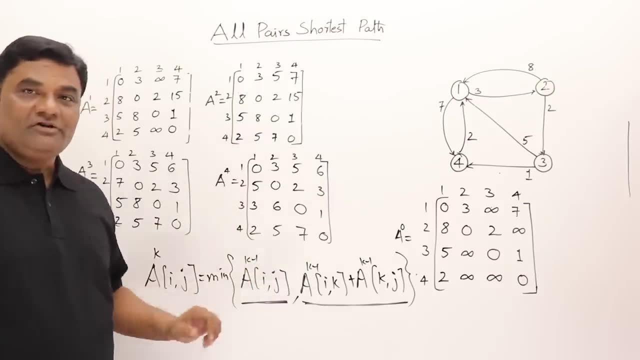 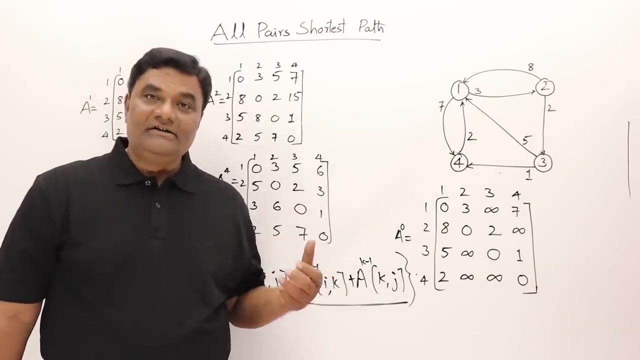 formula is used. See, I have first shown you the working. then I have generated the formula Right. instead of following the formula, I have deduced the formula. That's it. Now let me show you how the code looks like if I am writing the code. Now let us look at the code Every. 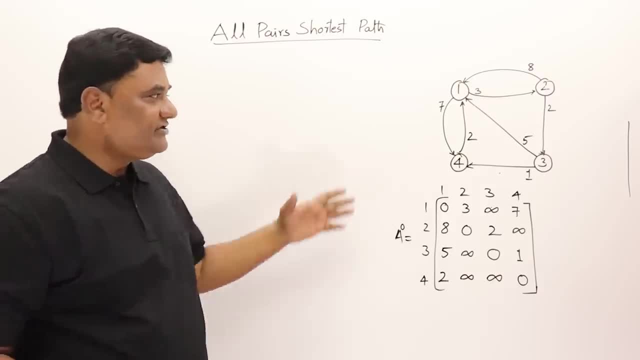 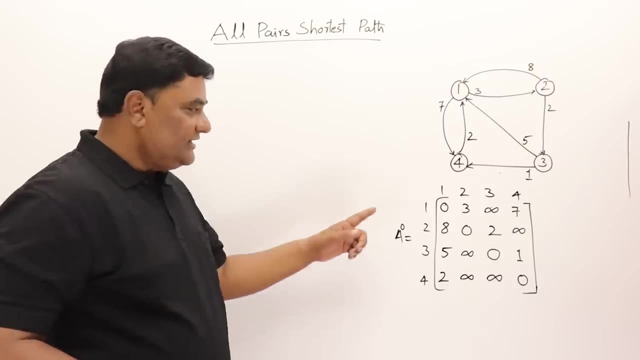 time I was generating the matrix. so how many such matrices I have generated? Four such matrices I have generated. Right now, for generating a matrix, what I am supposed to do, I should generate each and every term. So, total, how many terms are there? 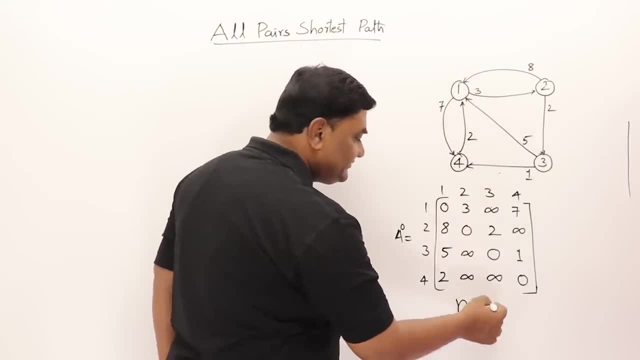 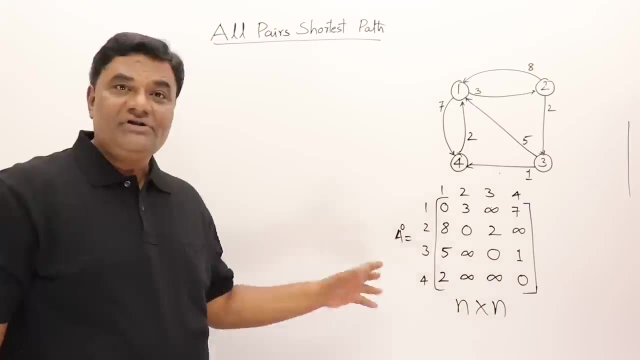 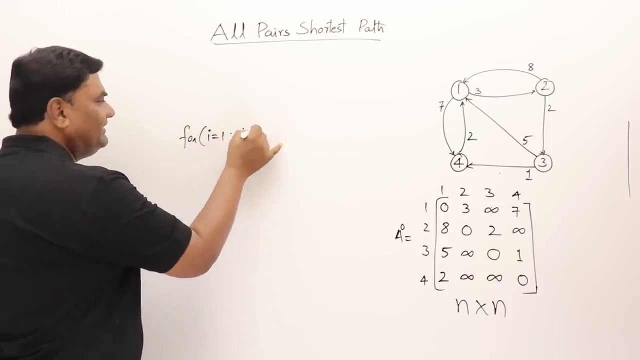 See, the number of vertices are four. So let us say n vertices. So the number of elements are n cross n. This is a square matrix. Now for getting all the elements of a square matrix I should have two for loops. So I will take two for loops, For i assigns 1 i less than. 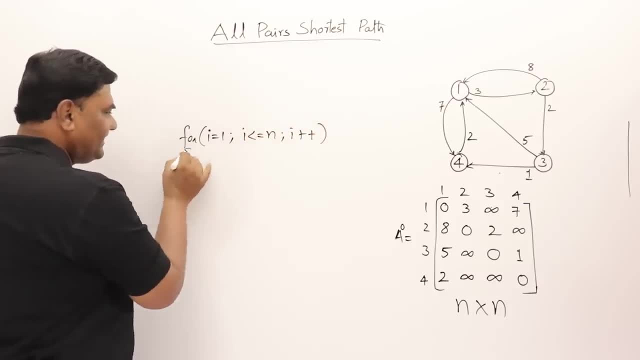 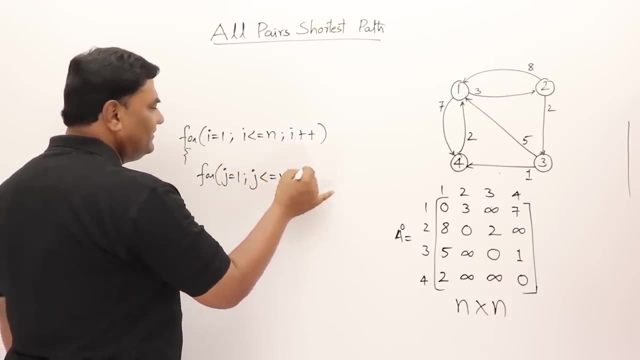 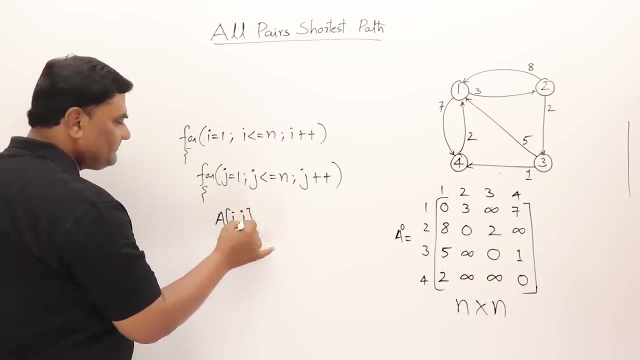 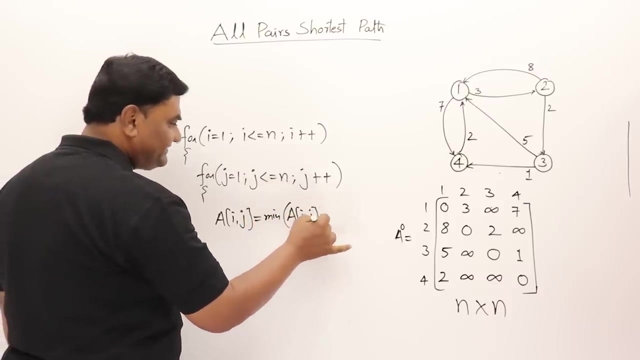 or equal to n i plus plus, and for j assign 1 j is less than or equal to n j plus plus And I should get the terms of a of i comma j as minimum of a of i comma j. that is existing matrix. as it is going to be a single instance of 2D array, In the single instance only I. 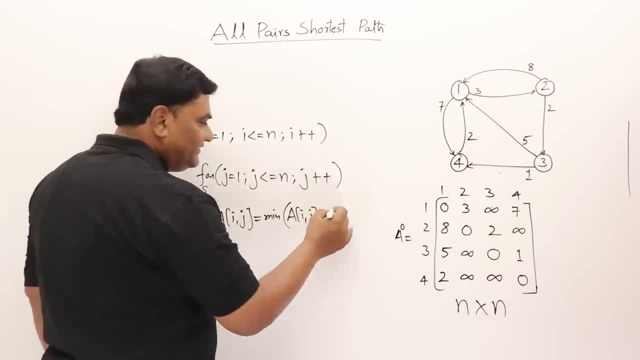 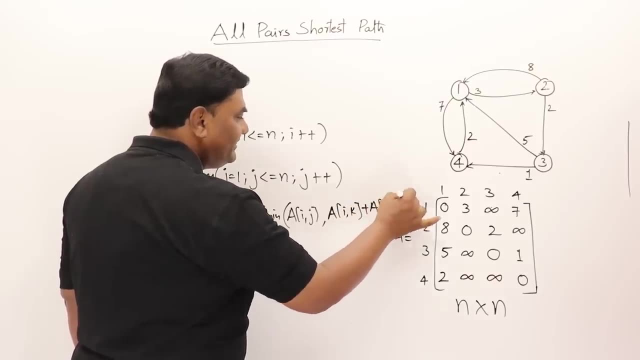 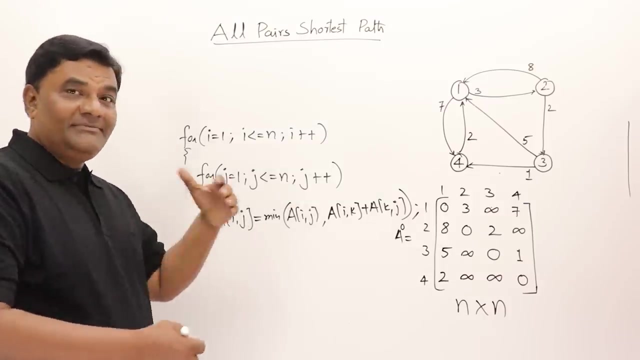 will be updating the values, So that's why this is same thing. Then a of i to k plus a of k to j. Out of this I should select any one of them, whichever is minimum. So what is k here? K will be changing the intermediate matrices, So this whole thing will generate just one. 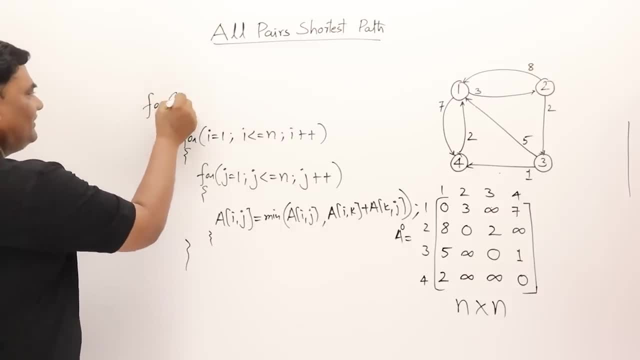 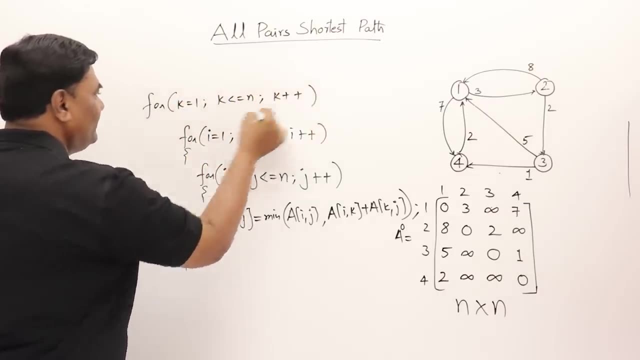 matrix and I have to generate all the matrices. So for k assign 1, k is less than or equal to n, k plus plus. Now, first time k will be 1.. So the intermediate vertex will be one all the time. Then k is 2..